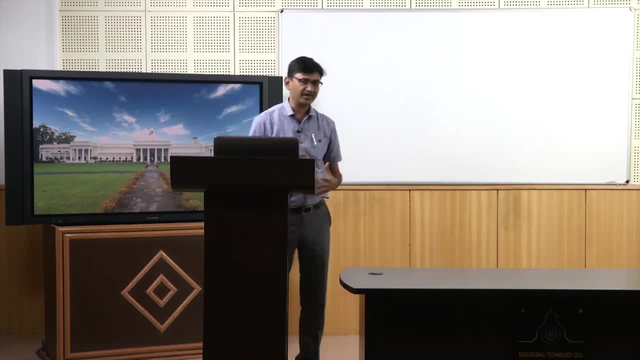 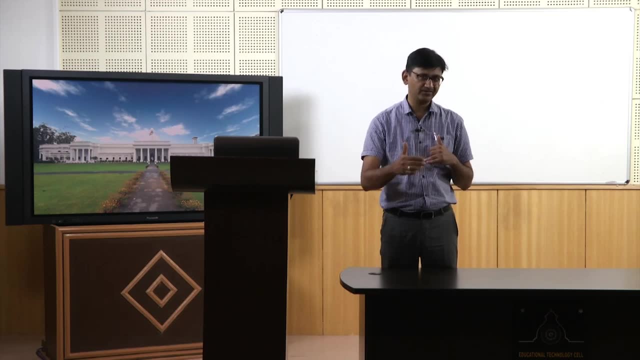 electrical magnetic properties. In fact, most of the metallurgy or study of ah, materials engineering is basically how to understand this defects, how to manipulate these defects and how to use these defects for our benefit. In fact, material without defects is a very boring material. okay, I. 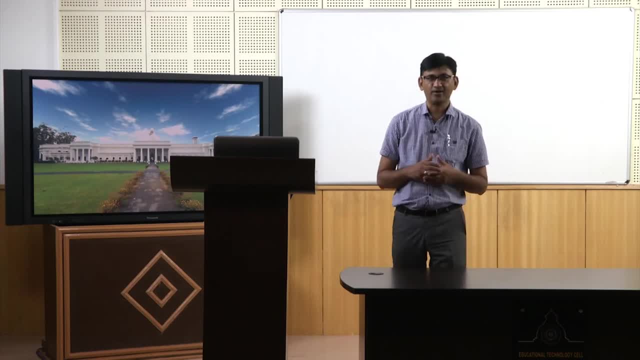 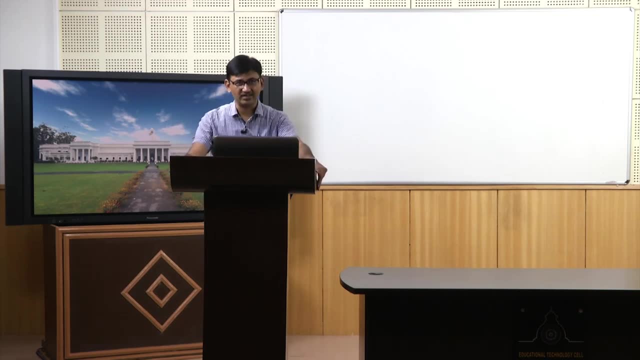 do not like a material which does not does not have any defect. okay, so any material. in fact, its use is based on. what kind of defects are there? and I can manipulate, I can tailor the properties of the material by manipulating the defects. okay, so defects are very important. they are not bad. okay, the defects are very. 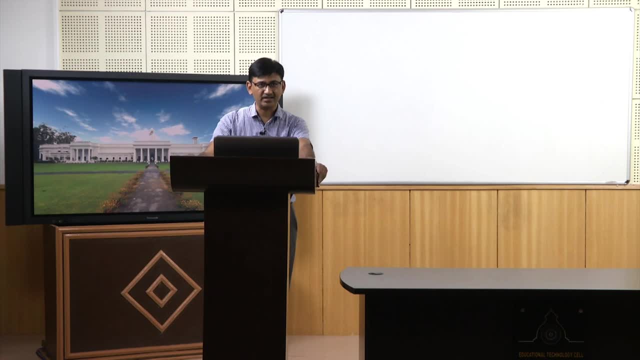 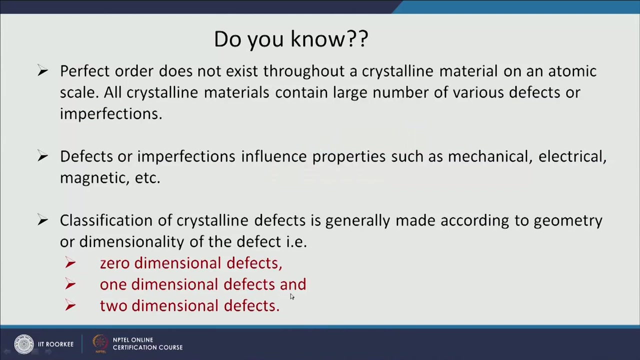 important for understanding of materials and as well as how I can design new materials by taking help of these defects. okay, If I want to quantify the defects, the defects are basically quantified based on their geometry and they are either called zero dimensional defects, one dimensional defects or two dimensional. 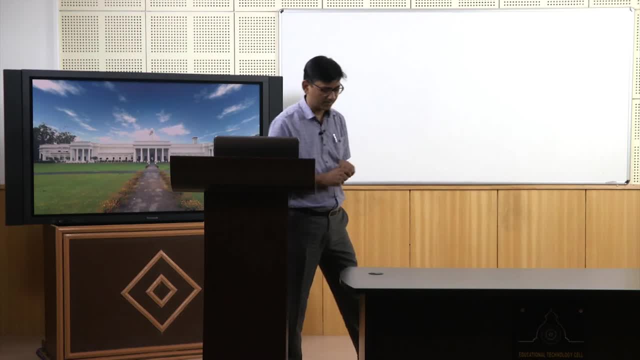 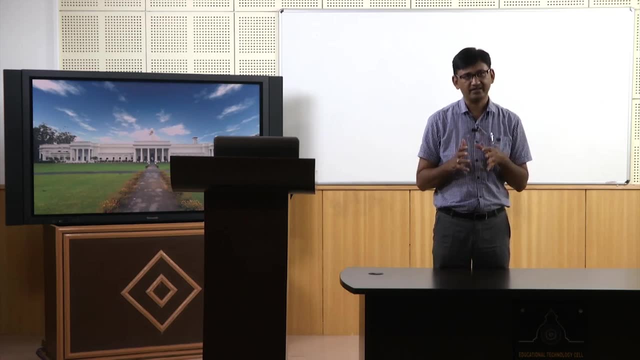 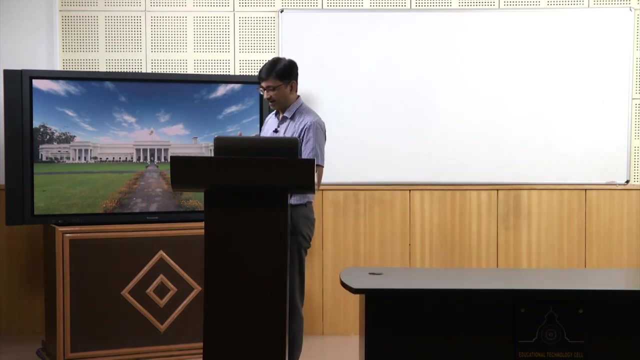 defects and volume defects also, But we are not. We are not talking about those defects in this particular lecture, because we are interested in the defects which are related to crystals, okay, or which are guided by the crystals, okay. so these are the 3 broad types of defects which are going to be there, okay, and we want. 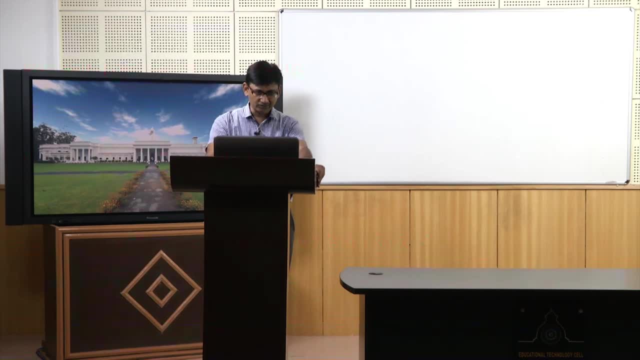 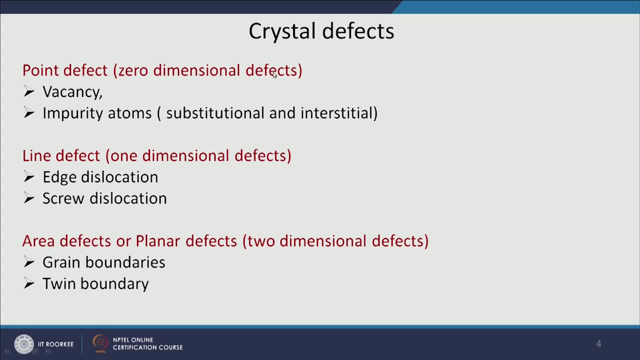 to study these defects again. in each of these category we can have different type of defects. for example, point defects, which is basically a zero dimensional defect. okay, it does not have, it is a point no dimension. okay, so in that you will have vacancy or you can have. 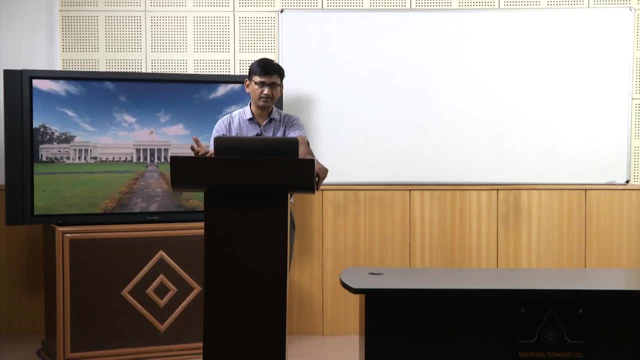 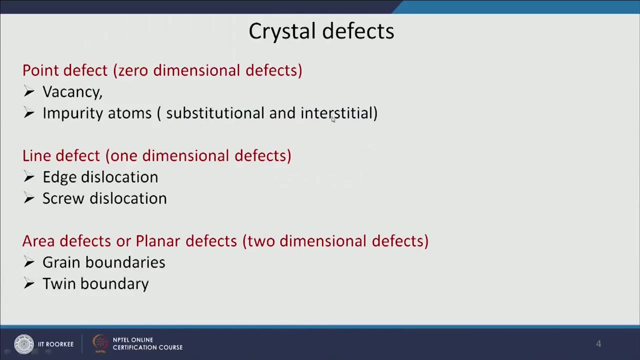 impurity atoms, okay, impurity, or sometime you can call them this, alloying elements. these are either substitutional or interstitial. we will see what do we mean by these two terms. Then there can be a line defect. Then there can be a line defect. 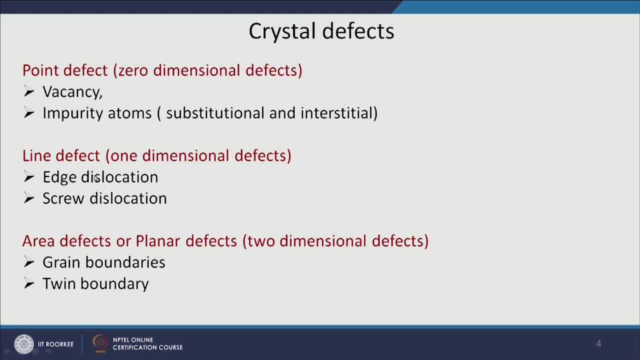 Then there can be a line defect, which is a one dimensional defect, okay, in that you will have edge dislocation or a screw dislocation- again, we will see what do we mean by these terms and what do we mean by dislocation itself. Then there will be area defects or planar defects, two dimensional in nature, okay, and 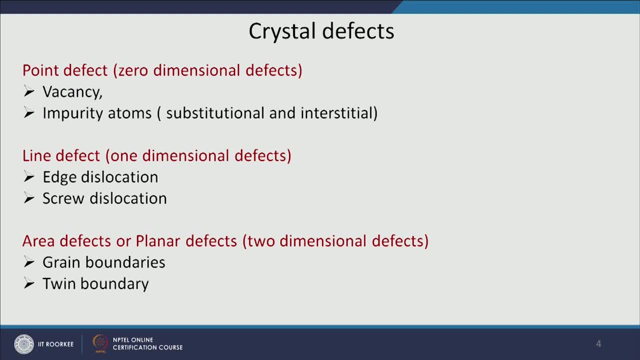 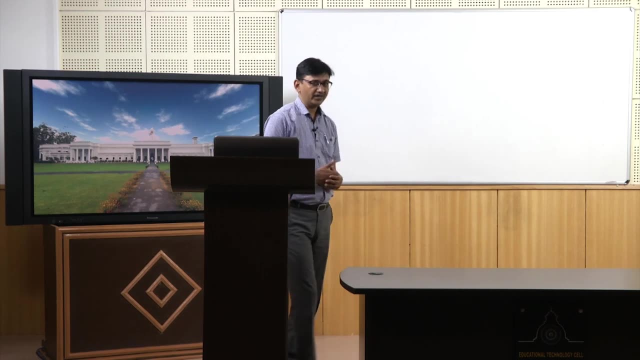 grain boundaries. we already now know this term: grain boundary, we have discussed that quite for some time, Okay. And another is twin boundary, okay. so again we will see. what do we mean by a twin boundary? okay, Now coming to point defects. you can classify them in these two types. actually, this encircled: 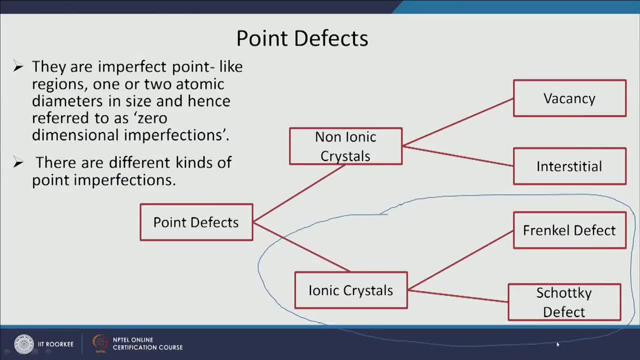 one I am not covering right now because these are mostly you will find in ceramics, okay, and they are of not interest to a mechanical engineer, as I understand. okay, So we will be mostly concentrating in a defects which you will find in a non-ionic crystal. okay, So basically point defects if you want to see they are imperfect. point like region, basically 1 or 2 atomic diameter in size, and that is why they are referred as zero dimensional imperfection. Okay, And there are different kind of point. 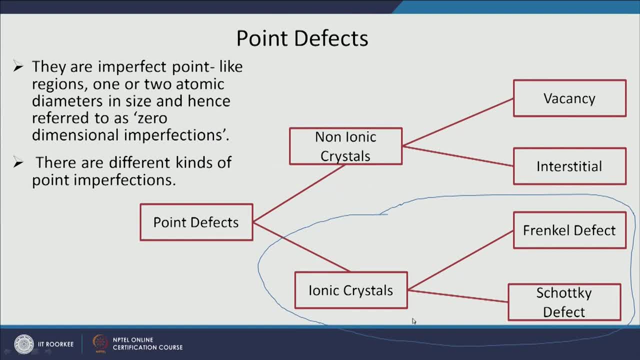 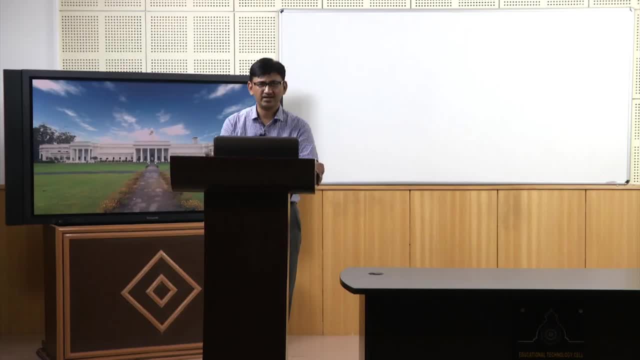 So there is non-ionic ionic in ionic you have Frenkel defects and Schottky, which we are not going to cover here, but if you are interested in any material science book you will be able to see these defects okay. 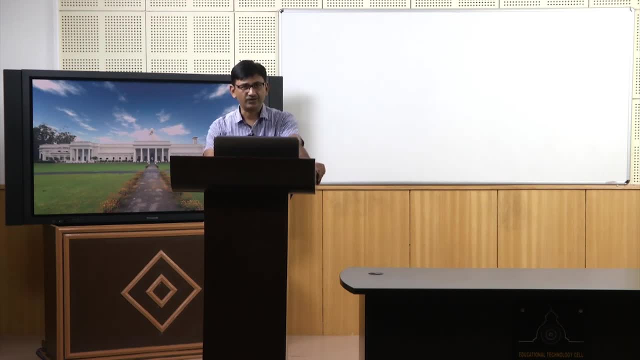 But we will be mostly interested in these two defects, which are of zero dimensional in nature. okay. So if you want to see vacancy, okay. Vacancy means in the regular arrangement. so you have lattice points, okay, and on each lattice point you should have an atom. 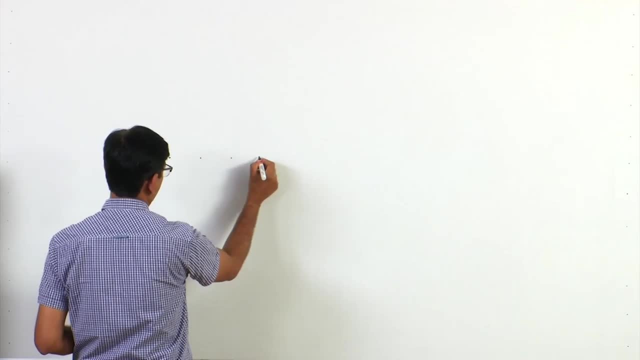 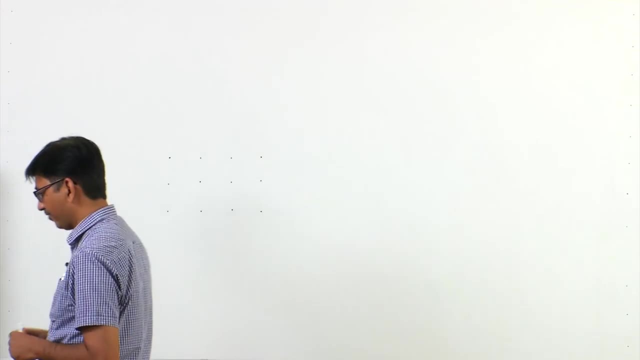 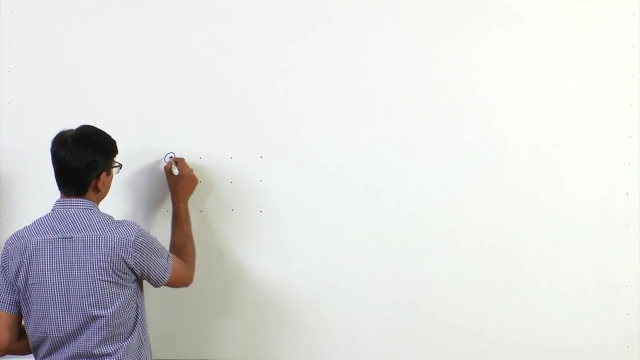 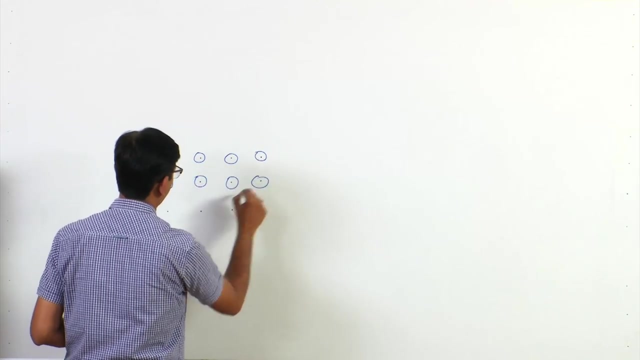 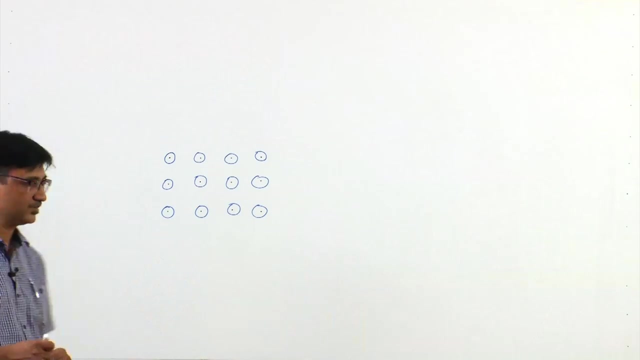 So suppose this is a lattice, okay, and of course, as we have already discussed in our crystal when we were discussing crystals, Okay, That on each lattice point, Okay, We are putting an atom here. Okay, So vacancy is when one of these atoms is missing from the lattice point. 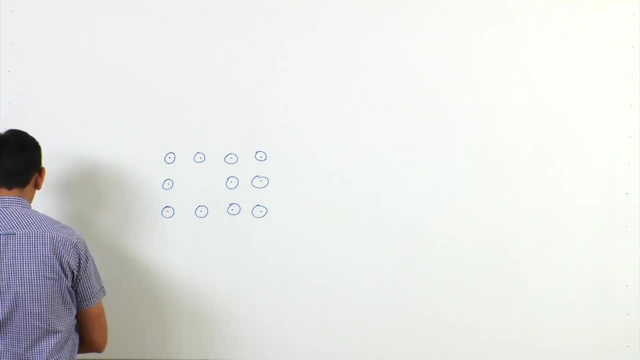 So, for example, this atom is not there. okay, So the lattice point is there, of course, but the atom is missing from that. okay, So there is a vacancy. now There is no vacancy. There is no atom there. okay, So this is called a vacancy, okay. 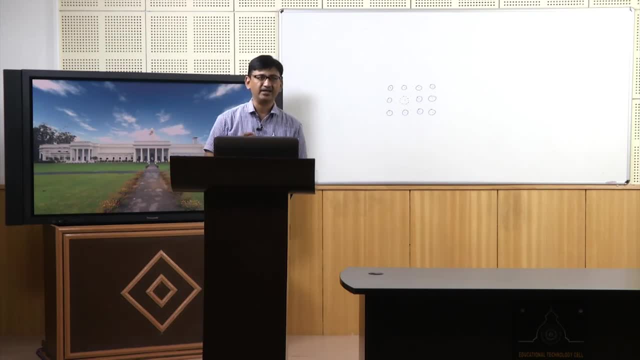 How they are created. They are created by thermal excitation. So when the temperature increases, what happens? all these atom vibrate on their mean position. okay, And in this process, sometime atom will get enough energy to break all the bonds from the surrounding atoms. 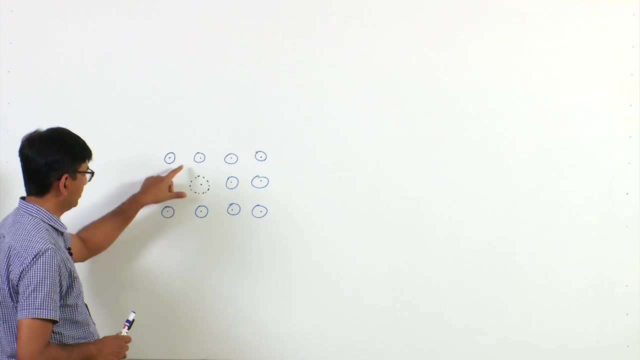 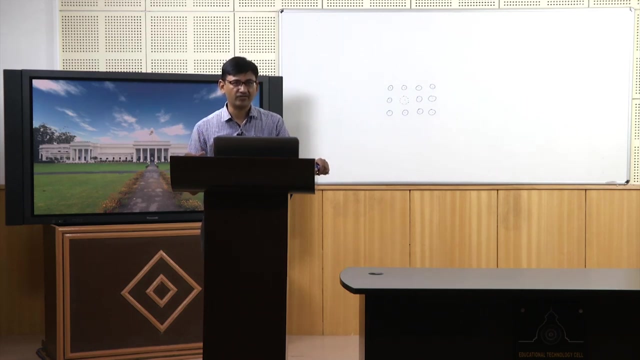 Okay, For example, was having bond with this one, this one, this one and this one- Okay. So it broke all the bond and came out of this lattice point- okay, and started roaming around- okay, and left a vacancy behind. So this is actually a temperature dependent phenomena. 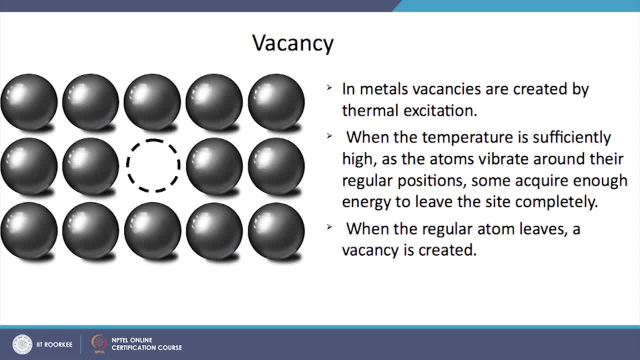 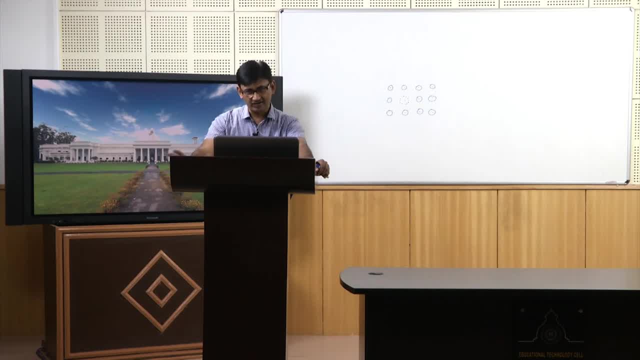 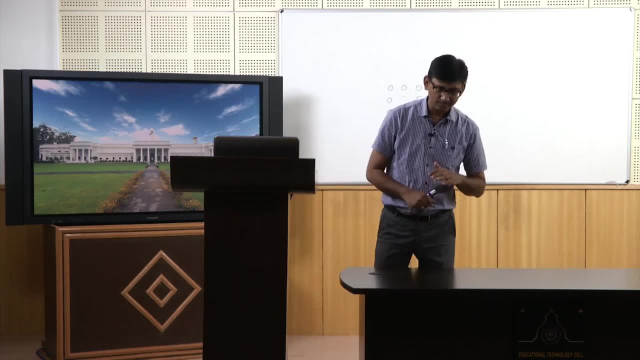 So when the temperature is sufficient and they vibrate, they get. So sometime they get acquire sufficient energy to break free, okay, And when they do that, it is called vacancy. Now, most important you can say quality of this defect which is called vacancy, is that 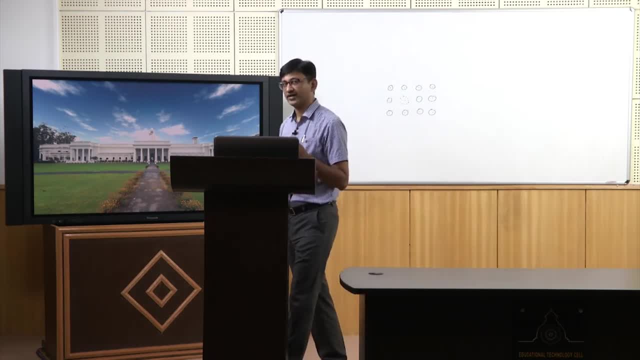 this is a thermodynamic defect. This is the only defect which is a thermodynamic defect. The meaning of thermodynamic defect is That it is- you can find it that- what will be the quantity of this defect in a particular material only by knowing the temperature. okay. 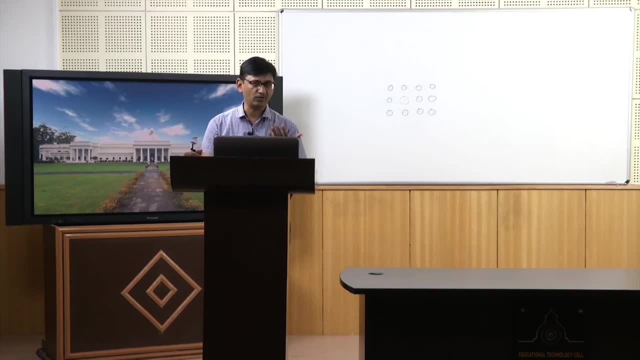 And it is dictated only by the temperature. So I cannot increase or decrease the number of vacancies in the material. okay, It will be dictated only by the at what temperature my material is at that particular point. Okay, So it is a function of temperature only. 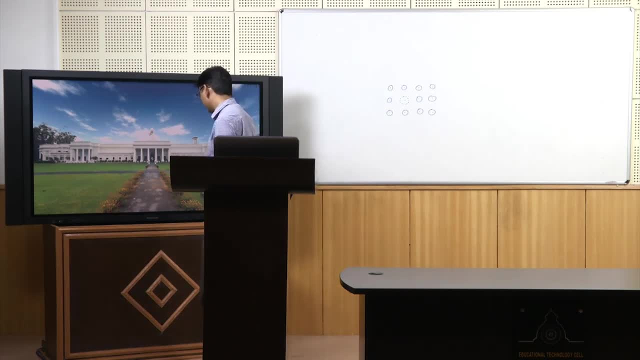 Okay, If you see other defects, these defects you can increase or decrease. okay, by doing certain, for example some deformation, or maybe by doing some kind of heat treatment, whereas in we can see it is only dependent on temperature and I cannot increase or decrease. okay, according to my will. 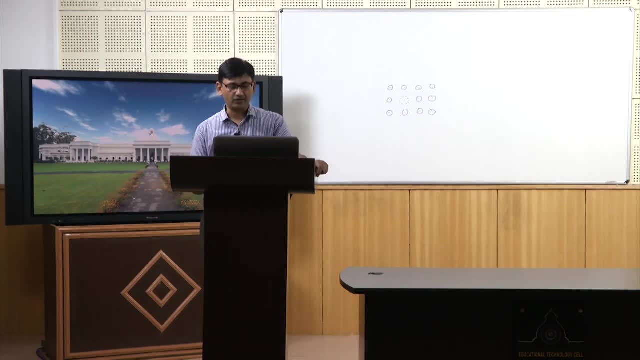 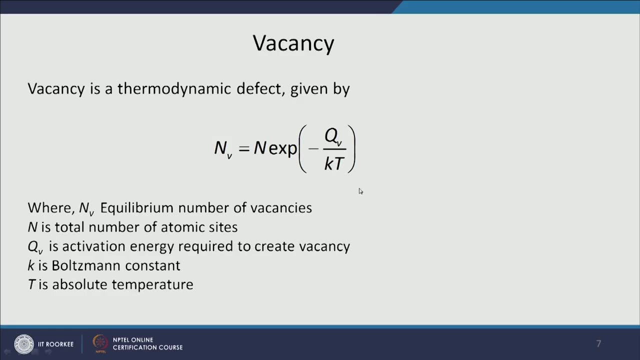 Okay, So this is the only thermodynamic defect, which is very important, okay, and the number of vacancies will be given by a relationship. Okay, So this is a relationship, a Arrhenius type of relationship, okay, where Nv is the number of vacancies. okay. 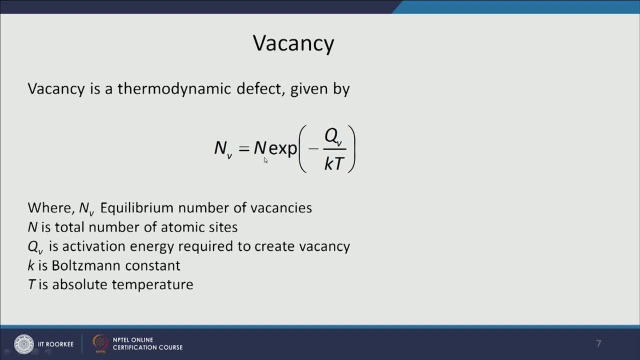 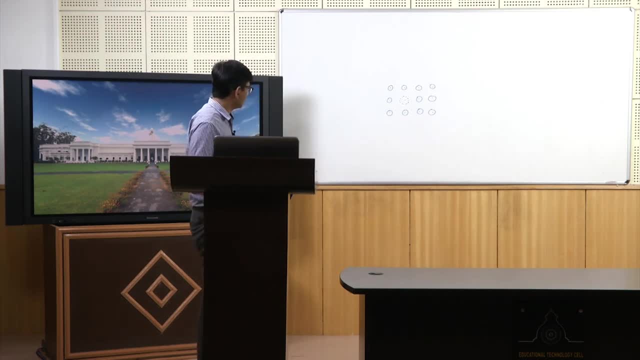 So in this case it is 1.. N will be the number of lattice points on which you should have atoms or atomic sites, which in this case, you can see that there are 12 sites like that. okay, and exponential, minus Qv is your activation energy, which is required to create the vacancy. 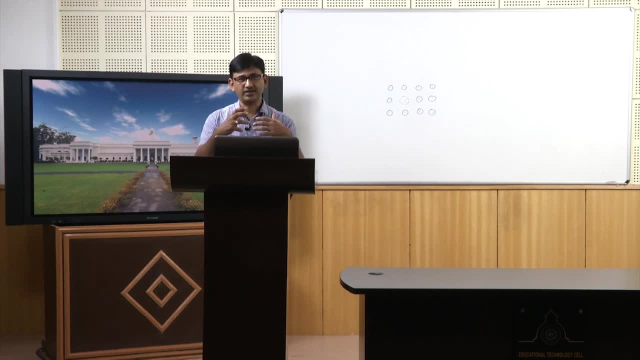 So basically it is related to the bonds. How much energy will be required to break all the bonds and take out the atom? Okay, K is Boltzmann constant and T is your absolute temperature. Okay, So if I want to know that, what is the number of vacancy will be there at a given temperature? 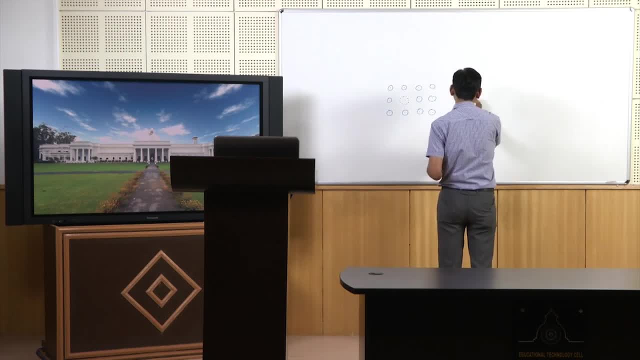 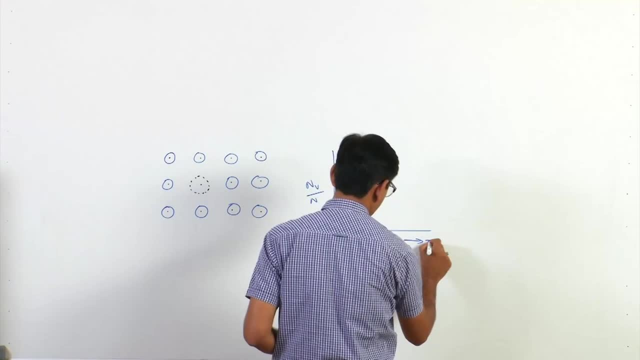 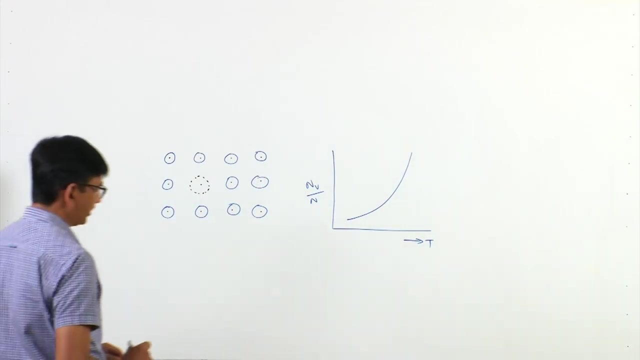 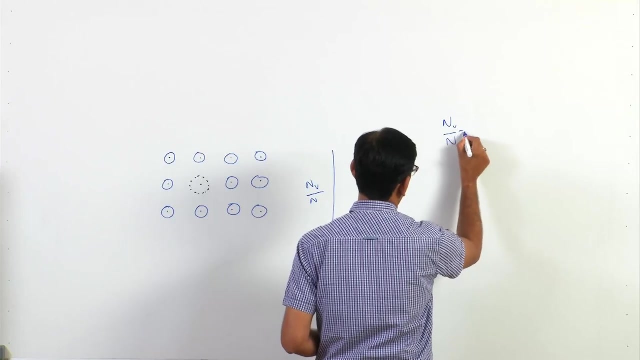 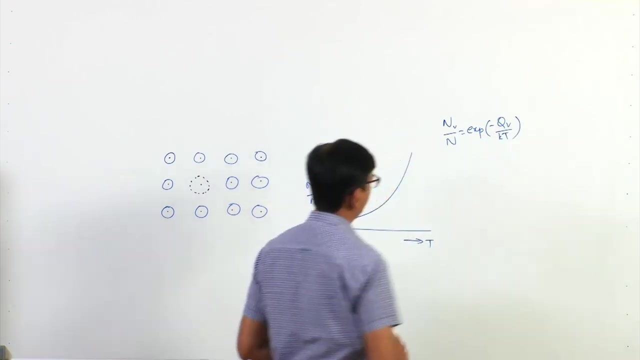 basically, if you this is exponential relationship, if I plot this relationship, okay, as a function of temperature, Okay, It will increase, something like this: Another interesting thing is that if I rearrange this equation, then it this equation will be like this: okay, and because this is an exponential equation, if I take logarithmic on both the 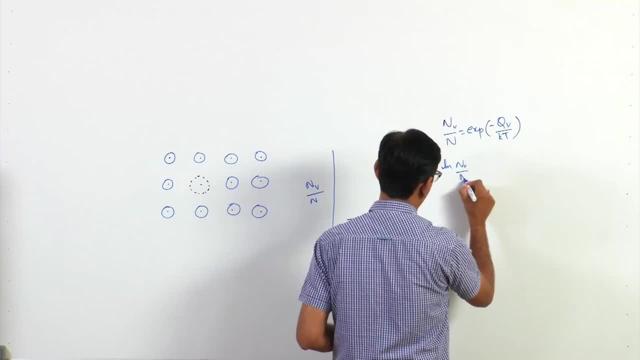 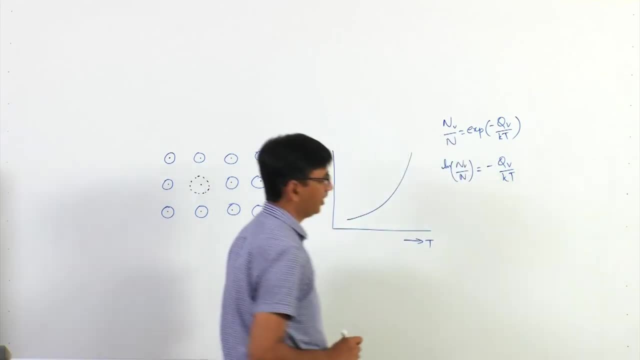 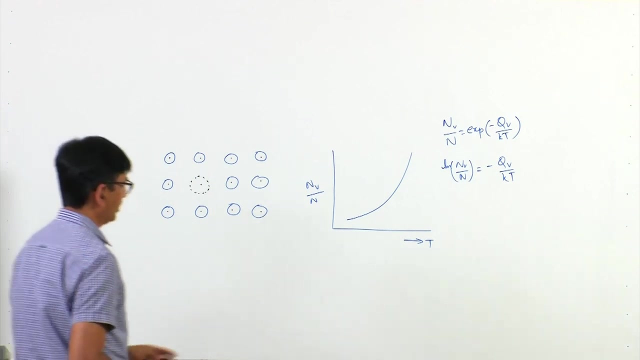 side. Okay, It will increase, something like this. Another interesting thing is that if I rearrange this equation, then it this equation will be like this. It will be, It will be. So it looks like a equation of a straight line: okay, where this is y. okay, this particular. 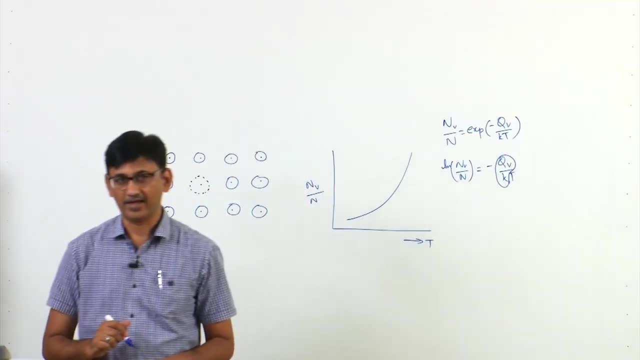 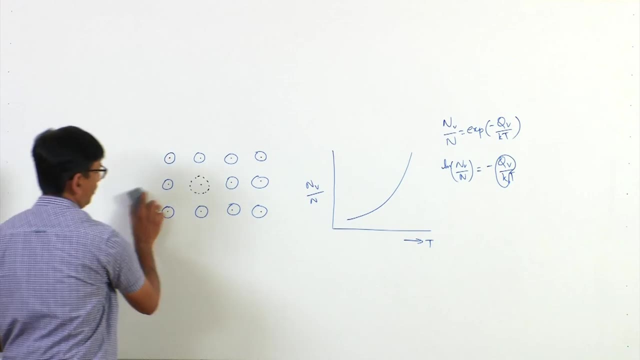 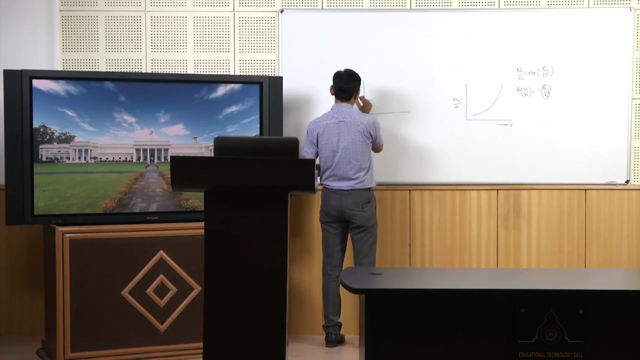 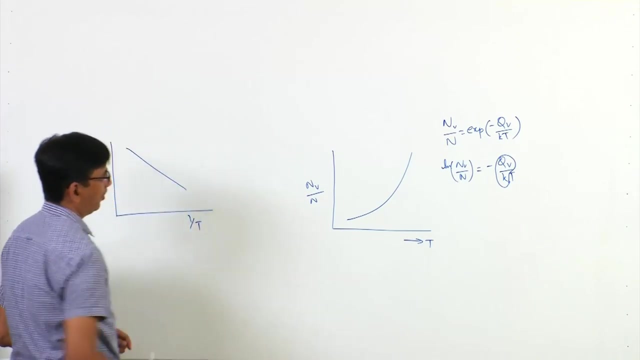 term is m and 1 by T is x. Okay, So if I plot now this, 1 by T Is A function of Logarithmic nv by n, so this is ln of nv by n and this is 1 by T. okay, then you will get a line of: 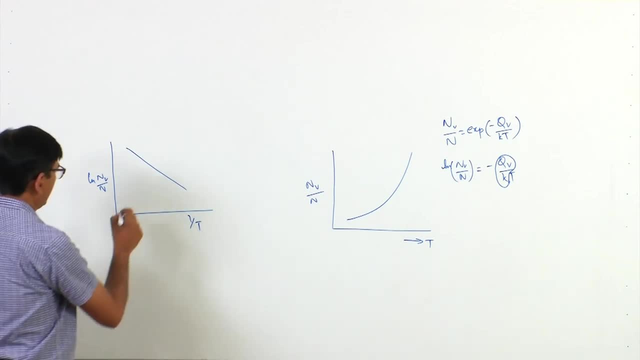 negative slope because there is a negative term there, and the slope of this line will be equal to qv by k. okay, so by knowing that how the number vacancies, number of vacancies, are changing as a function of 1 by T and by the slope, I can get what will be the activation. 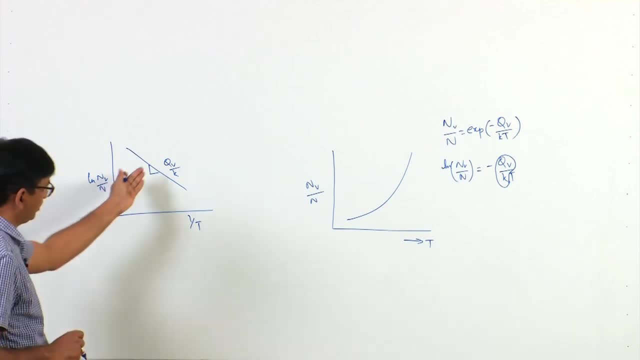 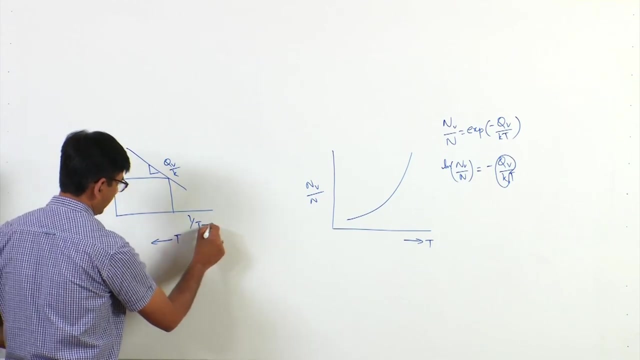 energy or, if I know, the activation energy. okay, I can tell you at a particular temperature what will be. the number of vacancies will be there. So 1 by T. 1 by T. if it is increasing here, that means T is increasing in this direction. so at a. 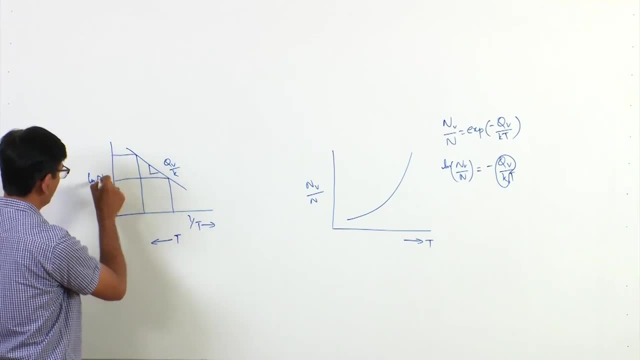 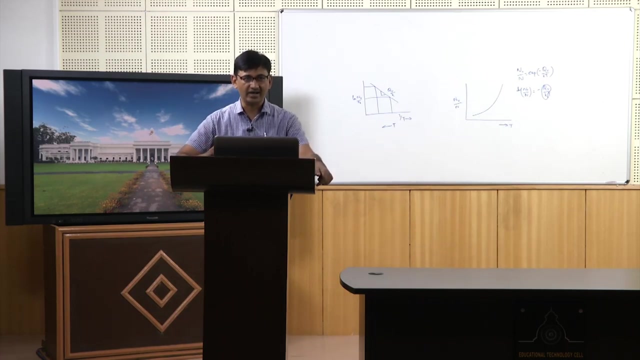 higher temperature, I will have more vacancies. okay. at lower temperature, I will have less vacancies. at 0 Kelvin, I will have no vacancies. okay. so at only 0 Kelvin you will have a material without any vacancies. at any other temperature, the material will have some vacancies. 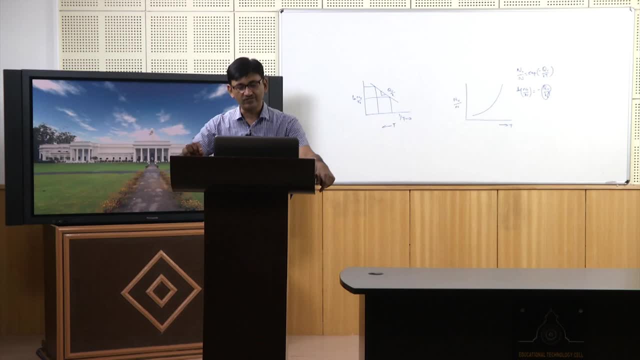 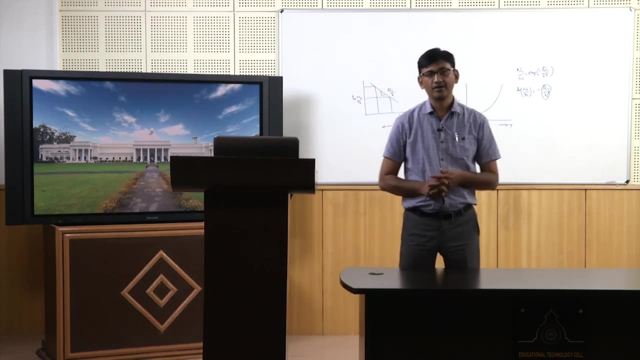 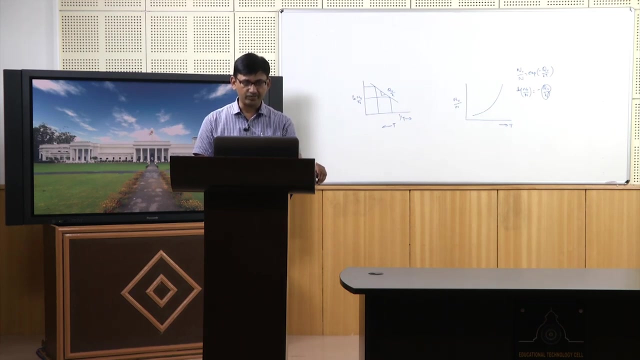 in the, And these are called equilibrium concentration of vacancies. okay. Then another type of point defects is called interstitial defect. okay, in which case an atom will come and occupy a interstitial position. interstitial means between these 2, 4 lattice. 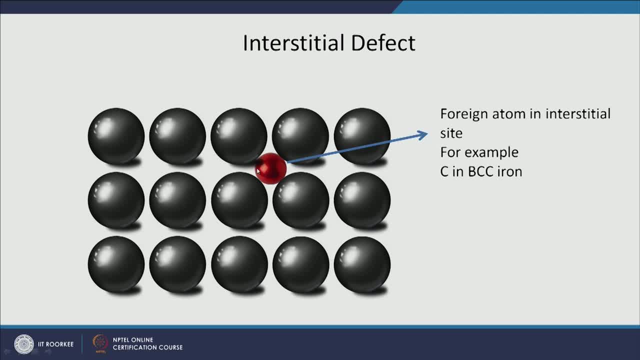 points there are atoms. on those 4 lattice points there is still some gap, is available for a very small atom to go and sit there, okay. So this is the point. So this site is called interstitial sites, okay, and a small atom can go and sit there. 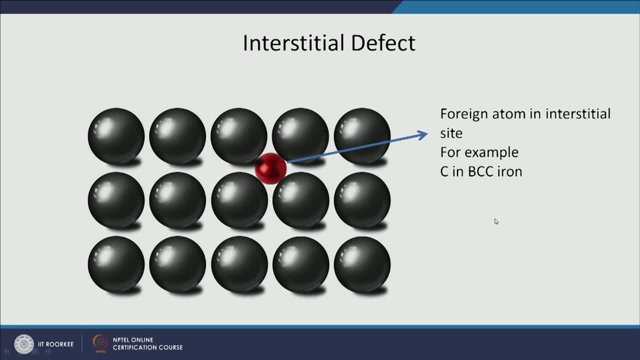 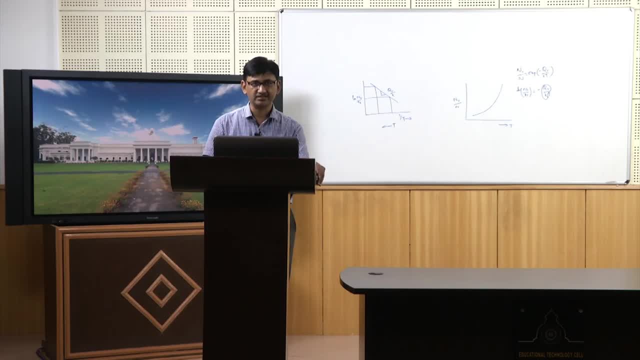 okay, for example, in BCC, iron. okay, carbon is a interstitial, an atom which is a very small atom. it goes and sit in the interstitial position. okay, Of course, this is a different arrangement than BCC. in BCC you will have different interstitial. 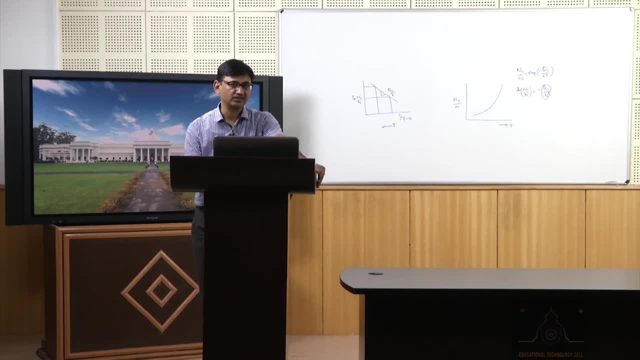 sites and the carbon will go and sit in those interstitial sites. So this is called an interstitial defect. so vacancies, basically you just take out an atom from its site. interstitial means a foreign atom will come and sit in the interstitial. 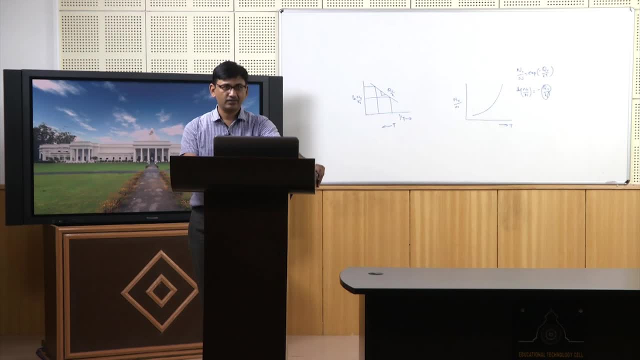 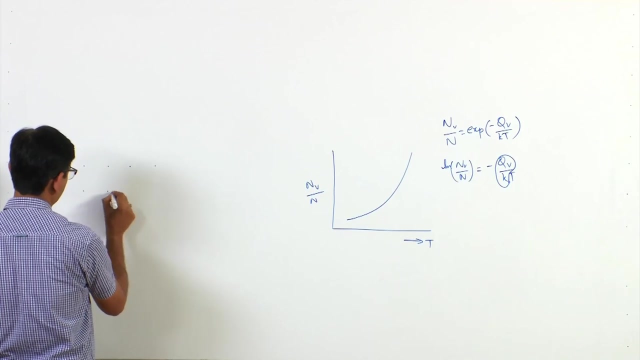 position. okay, Now, instead of vacancy you can also have a condition where a foreign atom comes and occupies the normal lattice site. okay, So earlier we saw that I can have vacancies. Okay, So suppose these are the lattice points and atoms are there on each of these lattice points. 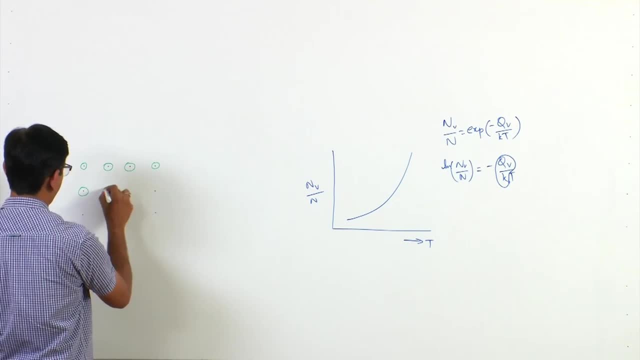 okay. So one case was that I said you can have a condition. You can have a condition where this atom is missing from this site. it is called vacancy. There can be another condition, okay, where another atom comes and sit in on this site, okay, and of course, the site of the size of another atom, which is foreign atom, which is 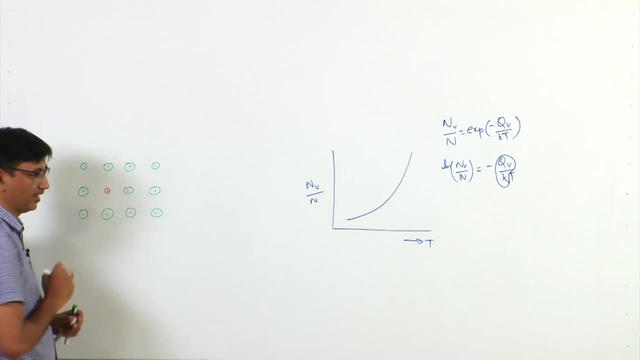 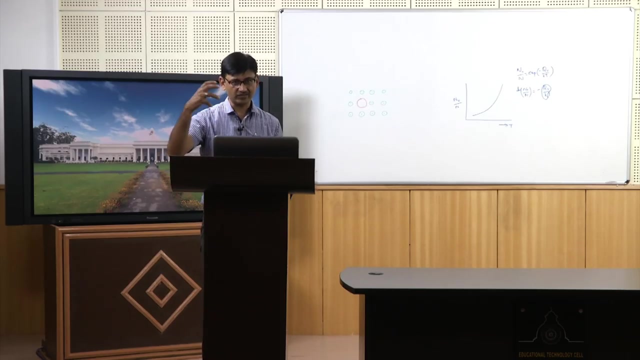 coming can be small than the earlier one, okay, or it can be a bigger one, Something like this: okay, It is coming and sitting, So it is substituting the parent atom, which is already there- host atom. okay, and it is going and sitting there. 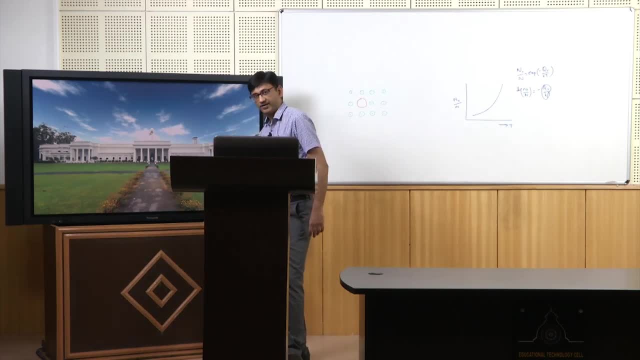 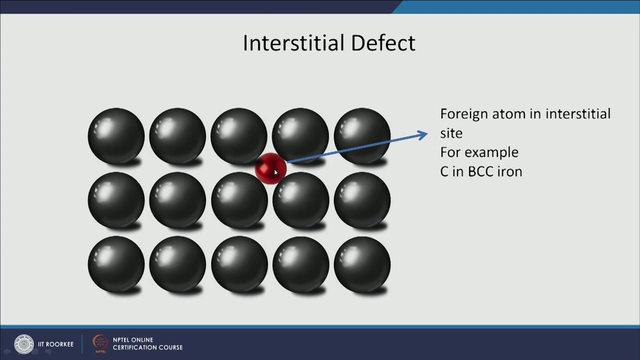 That is why it is called substitutional defect or substitutional impurity atom, because it is replacing the host atom and sitting, whereas in interstitial case you can see all the lattice sites are occupied Host atom and the impurity atom is occupying the interstitial position. 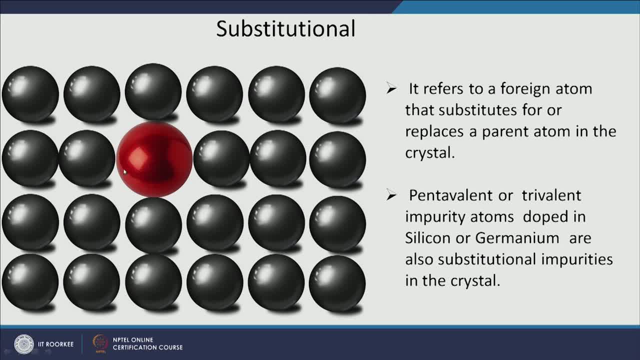 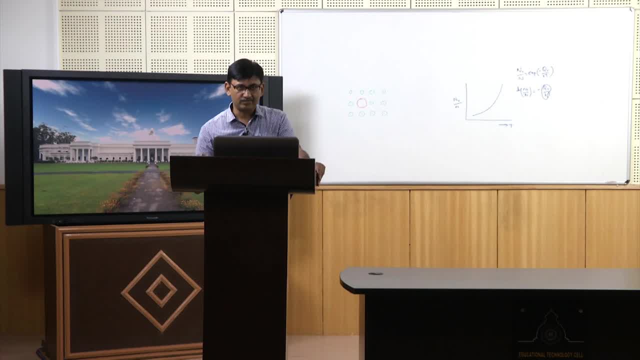 In case of substitutional, it is occupying the, it is taking the lattice site occupied by the host atom and that is why it is called substitutional defect or it is called substitutional impurity atom which is occupying this particular position. okay, and pentavalent and trivalent. 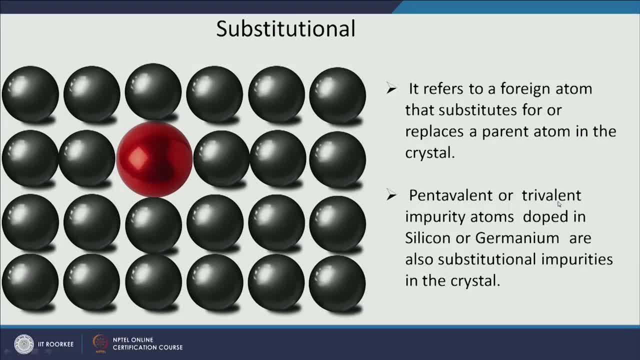 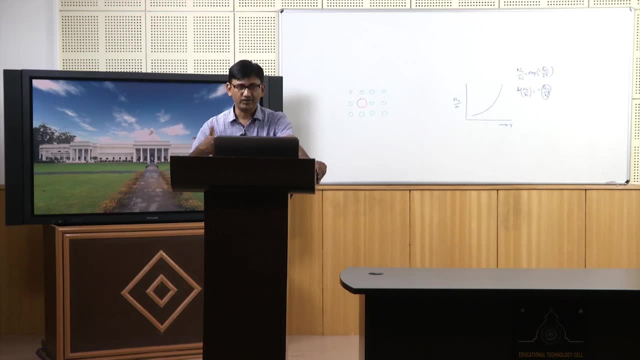 impurity where we do prepare a semiconductor: Okay. When we dope silicon or germanium by either pentavalent or trivalent impurity, okay, they occupy this substitutional positions only. okay. By doing that we prepare a semiconductor either P type or N type, okay, depending upon whether 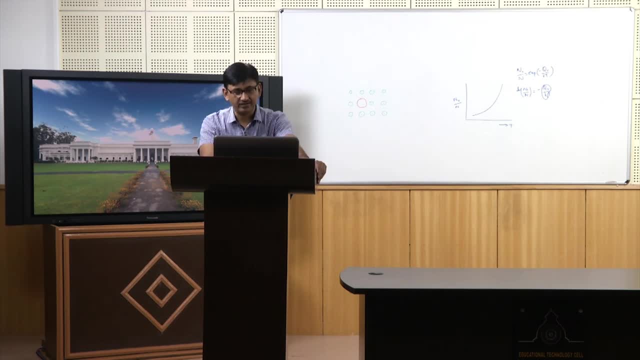 we are adding pentavalent or trivalent impurity atoms. okay, So this is one of the example where you will find a substitutional impurity Occupying this, occupying the regular lattice site. Then one of the very important type of defect which you will find is called dislocation. 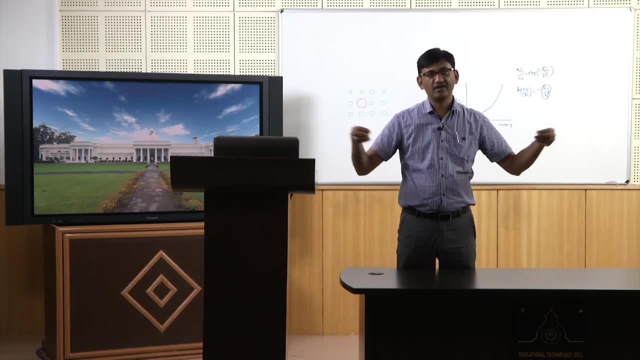 and this is a linear defect, or which will have one dimension. okay, So it has a dimension where the length of the dislocation will be a one dimension and there is no other dimension to that. okay, So this is called a linear defect. 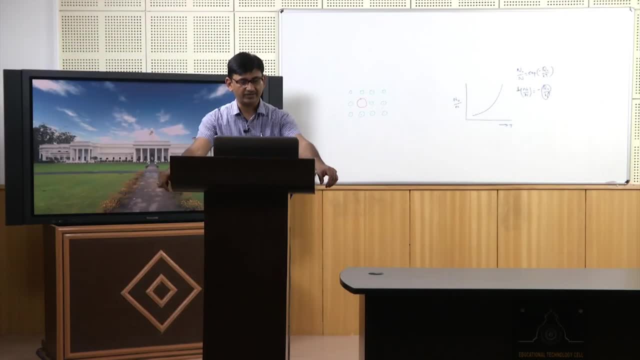 Okay, Because it has one single dimension. actually, how people started thinking about this particular defects? okay, has a nice kind of a story around it, Because when people were looking at this plastic deformation, that how material deform, okay- they found out that the two atomic planes- okay, or two layer of atoms, actually have a 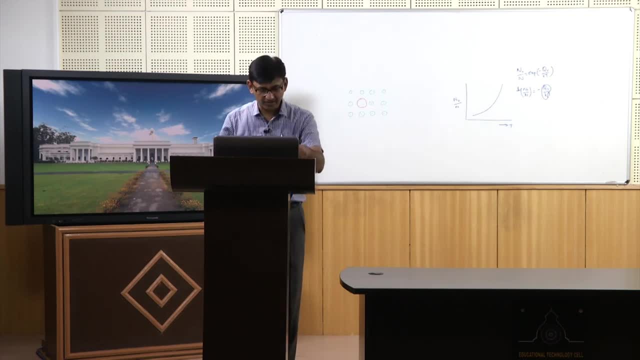 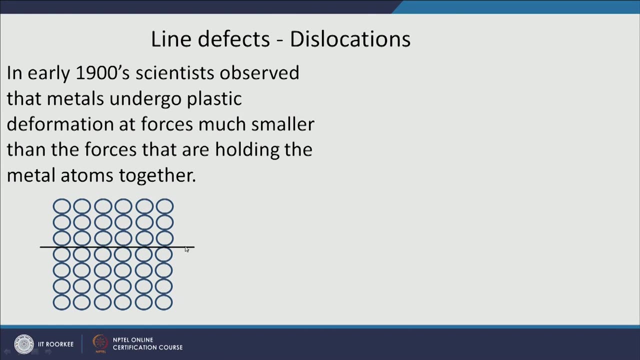 slip over a particular plane. okay. For example, I can show you this slide, this animation here. So you have arrangement of atoms. okay, and I have shown a plane with a black line here. okay, and I am applying the shear stress on this particular arrangement of atoms. okay. 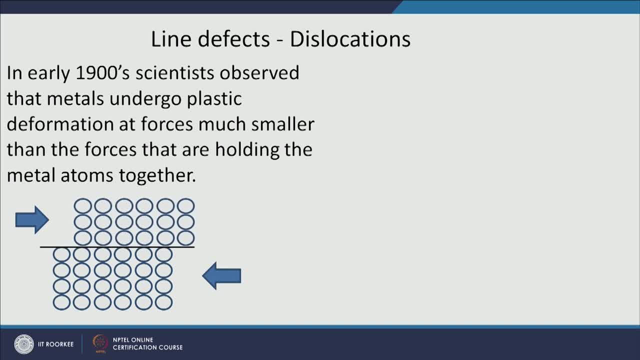 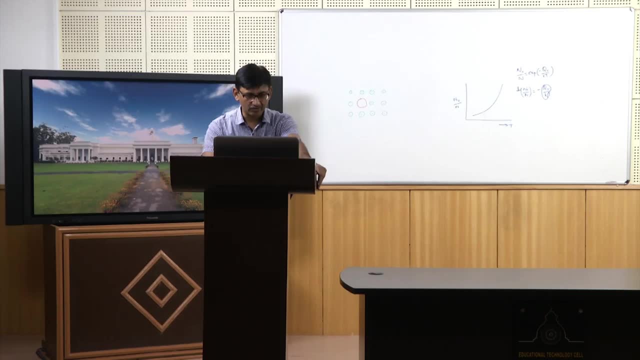 and because of that there is a sliding of atoms. okay, so upper half of atoms are sliding over lower half, So you can see that in the previous arrangement there was some bond between all these atoms. let me go back. So you have all the bonds between these two atoms and this will be along the whole plane. 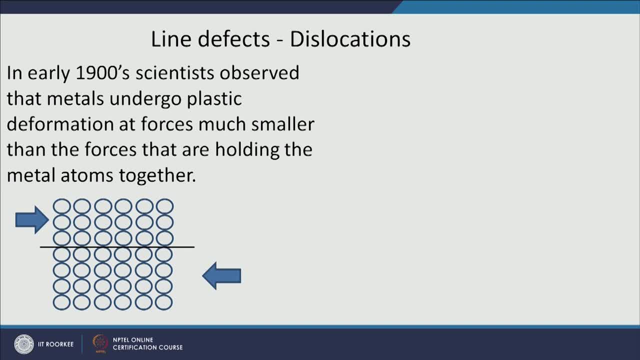 okay, and when I am applying the shear, then all these bonds for all the atoms are going to break and they will form new bonds. okay, So all has to break and we have to find new bonds. So all has to break and we have to find new bonds. 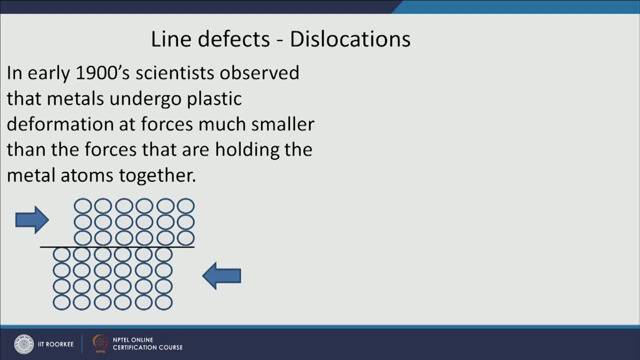 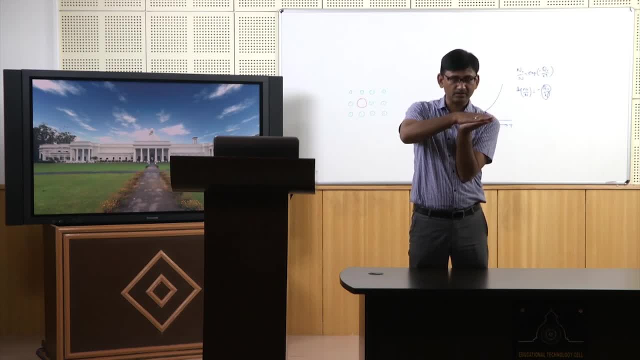 Okay, Okay. So all has to break and we have to find new bonds. Now the problem with this whole scene here is that we are simultaneously breaking all the bonds and creating this slide of atoms, okay, or this sliding of atoms, and this is going to require hell lot of energy, okay. 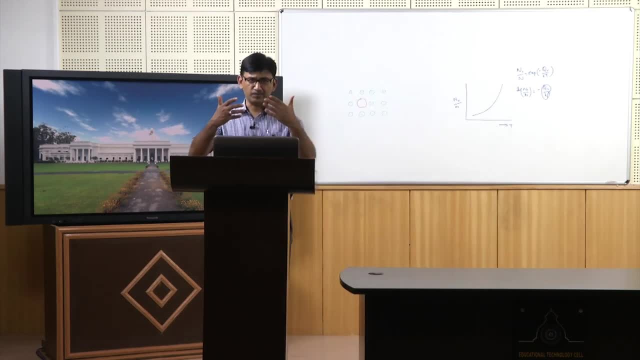 So the forces which people found out were much lower than what you will calculate by doing this kind of movement, okay. Okay, So all the atoms are taking part in the sliding process together. okay, So all bonds will be broken and new bonds will form. okay, and this will require very 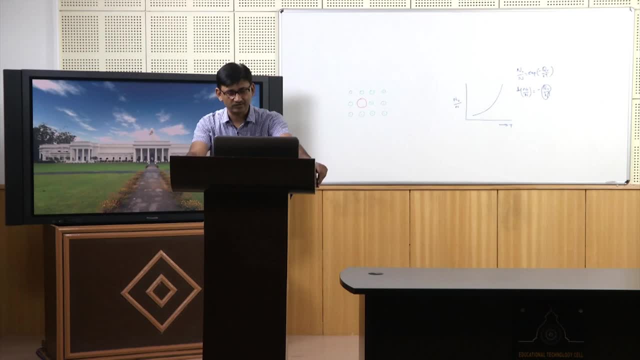 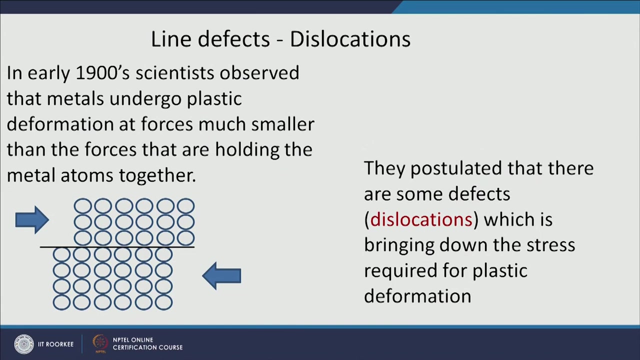 high energy, okay, and very high force, but the measured force was much lower than that, okay. So then people thought, or they postulated, that there may be some defects in the material, which is helping us to deform a material at a very low force or at which requires a lot. 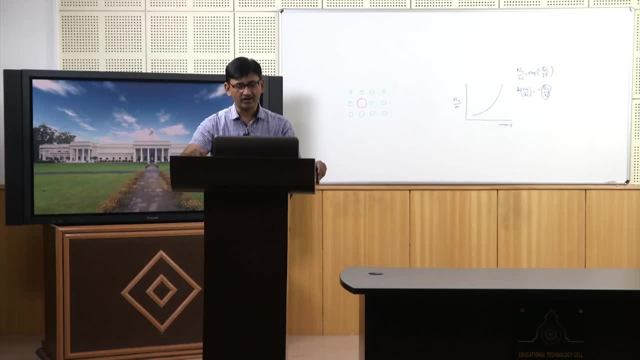 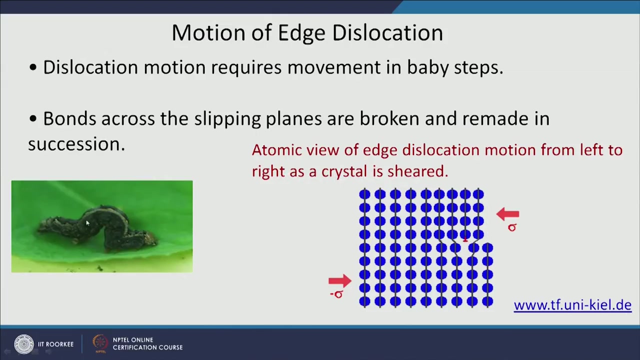 of which require much lower energy. okay, and they started calling it as dislocations. okay, and why this dislocation require less force. I will show you in the next slide. You can see a nice image of here of a caterpillar. okay, how it is moving. 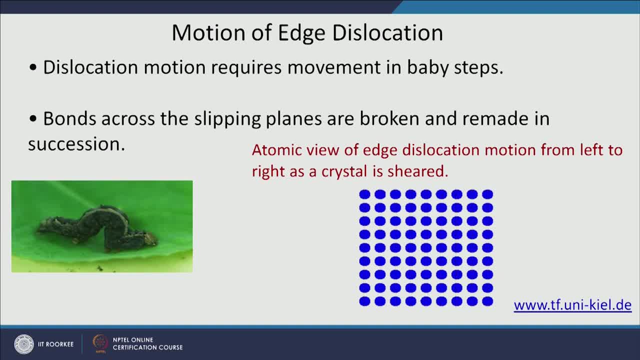 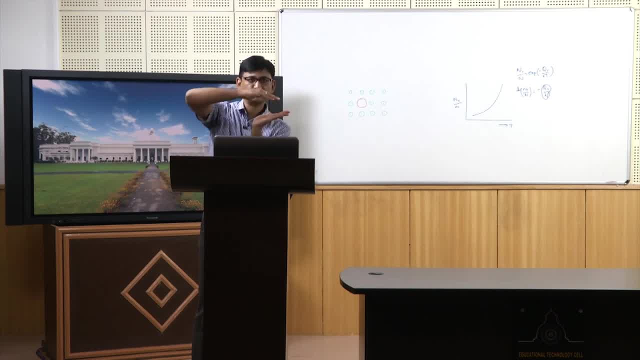 So a caterpillar will never move like this. okay, what it does, it moves in a step like that. okay, So it raises its body away from the earth and then it moves. okay, So that the idea is that it should have low, very less friction or very less contact with 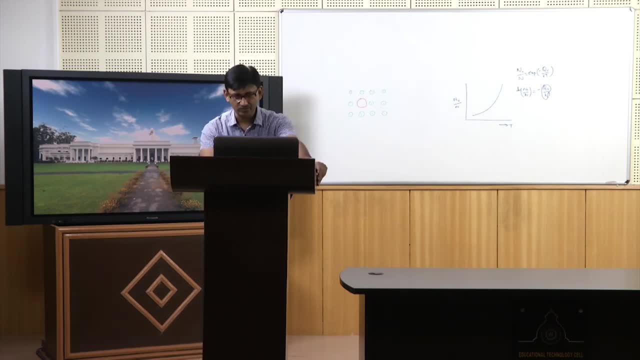 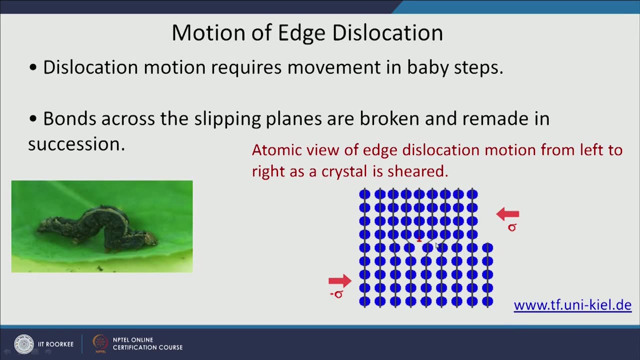 the earth when it is moving. okay, and that is very nicely shown in this particular animation. I have taken this animation from this particular website. okay, you can see that in each step, one bond is broken. okay, So I am applying shear, I suppose, to the previous step. 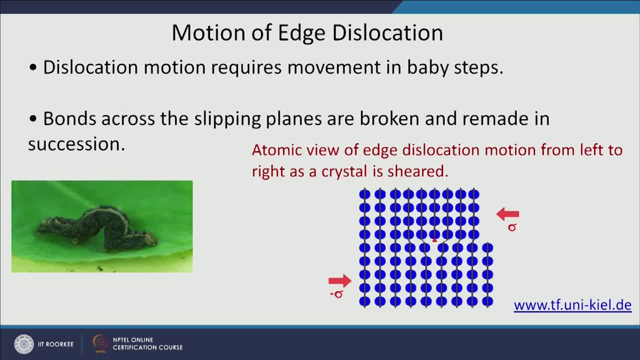 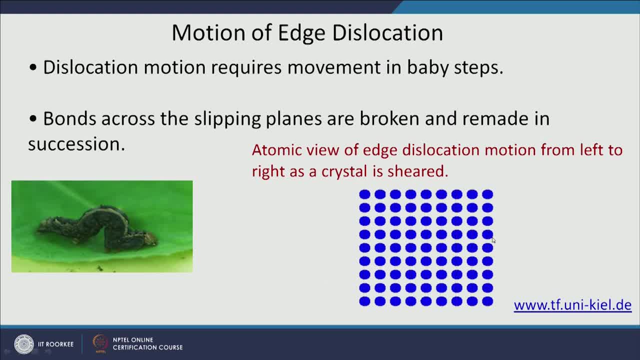 you can see that when I am applying the shear stress here: okay, the bonds are broken one by one, So you create this and then you create the step at the end. okay, So, instead of one big step, what we are doing? we are moving or we are creating this step. 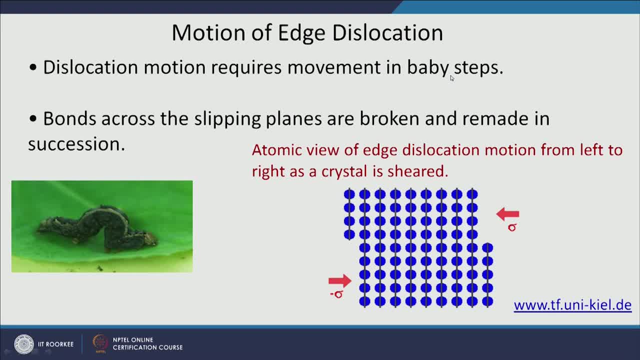 by small, baby steps, one by one, okay. So, for example, if I am applying this material at the end, So let us say it is this, this is the silence layer, And this will give. this will require much less force than what is required if I slide all. 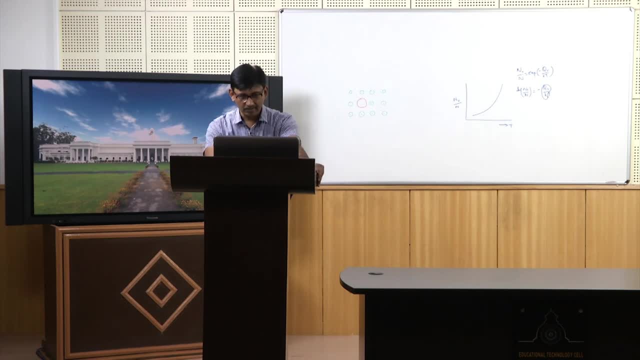 the atoms together. okay, and this sliding is helped by the creation of dislocation in the material, So that you can see by this red line here which is depicting the dislocation which is helping and creating the step at the end. okay, Now, of course it was not visible. 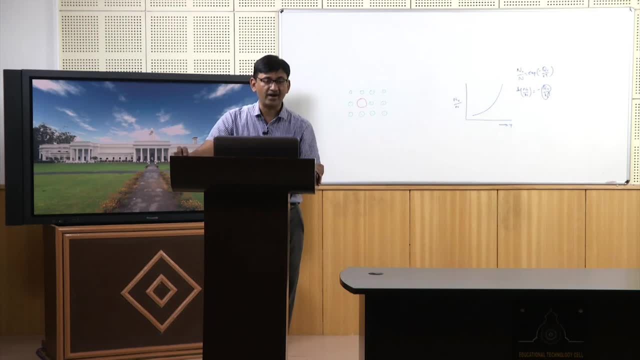 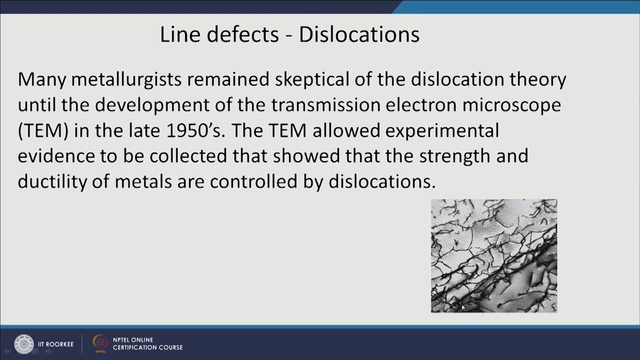 it was initially thought about that this type of idea is there and later on, when electron microscopy was invented and transmission electron microscopes were developed, then people saw that actually this is the case and you can see, this is a nice micrograph and you can understand the. actually the scale length is not there, but these are at nanometer scale. 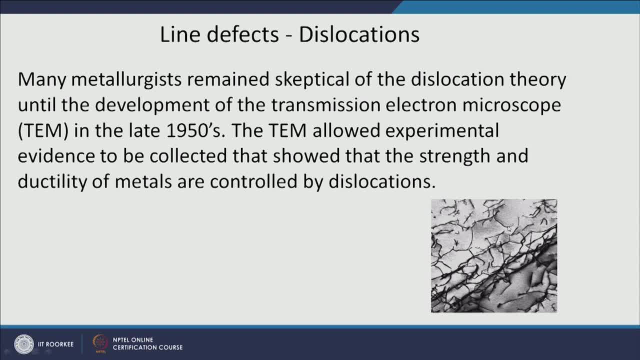 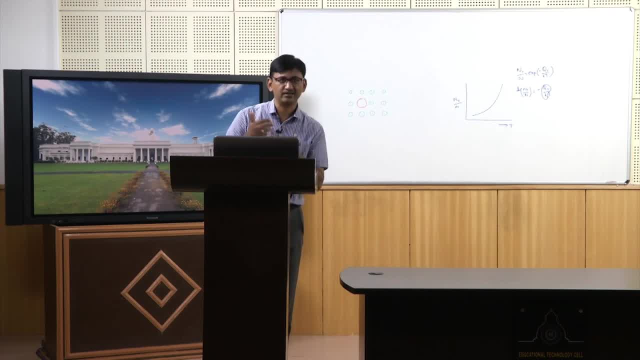 and all these lines which you see are dislocations. these are all dislocations and people did lot of experiments that if you do lot of deformation this dislocation density increases. if you do any link, this dislocation density goes down. so by that they could understand that. 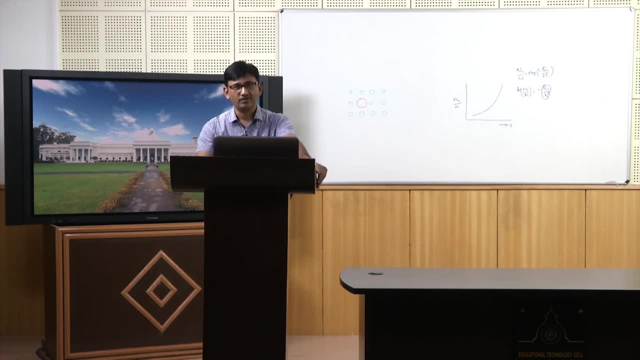 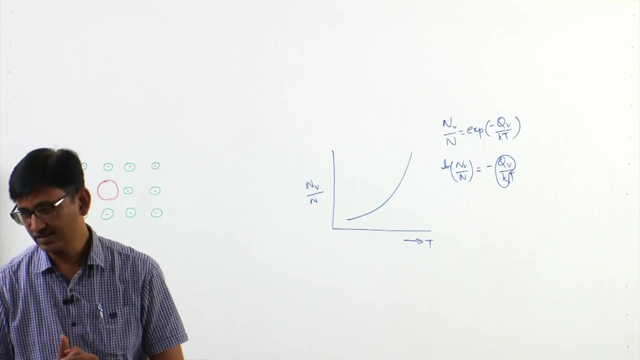 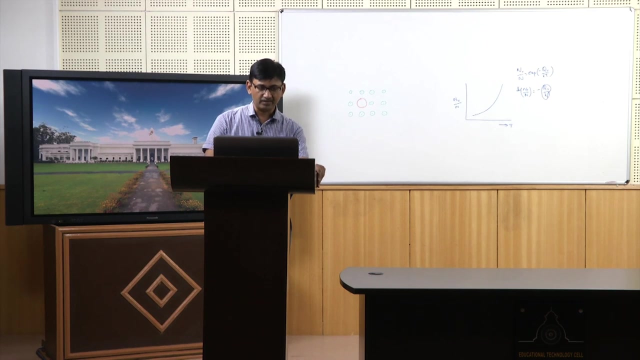 this. dislocations are the main source or main driving vehicle for deformation, and that is what they and they control the strength and ductility of metals. Now I can divide this dislocation also in two. I can classify them in two ways. one is what we call as edge dislocation. in case of edge dislocation, the Berger vector is perpendicular. 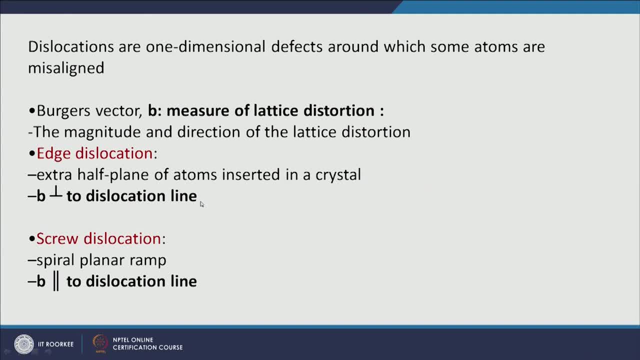 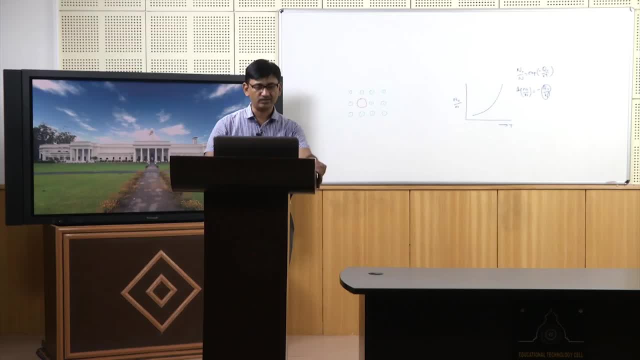 to dislocation line, we will see what do we mean by a Berger vector. and in the screw dislocation the Berger vector is parallel to dislocation line, so you can have these two type of dislocations based on how the Berger vector is with respect to the dislocation line. 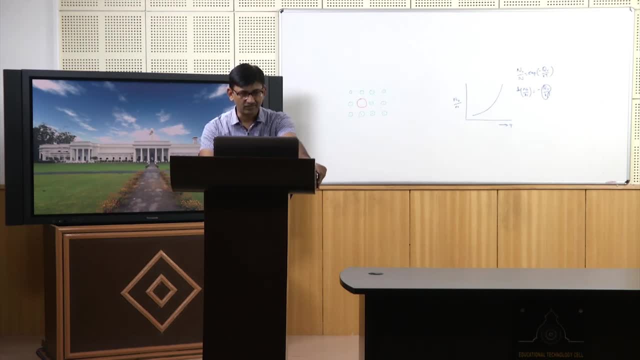 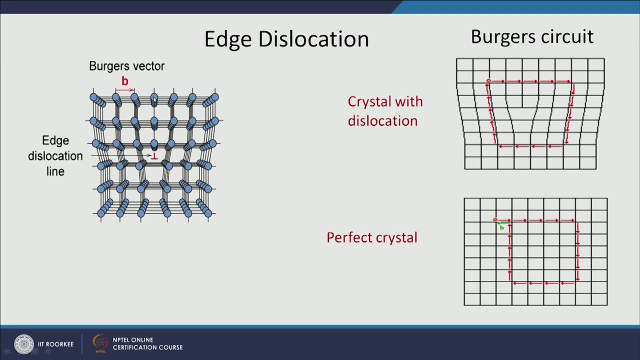 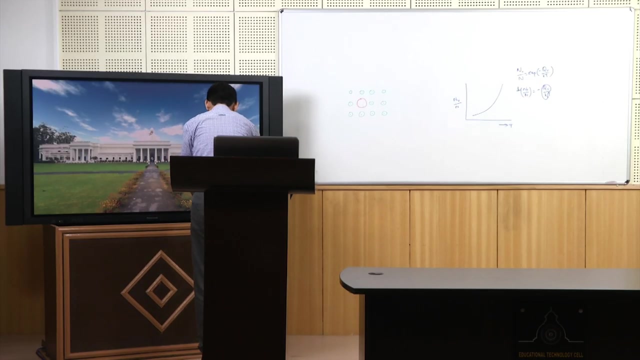 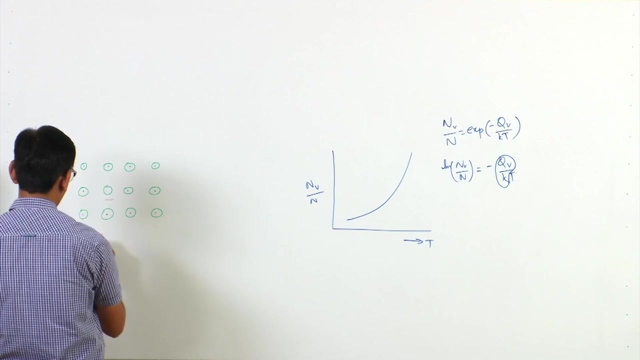 So, for example, here you can see a nice wire frame kind of structure. so a regular arrangement was there. but you have inserted a half plane in the arrangement. so initially you can see, you can see that I have a simple arrangement like this. maybe one more I can put here. 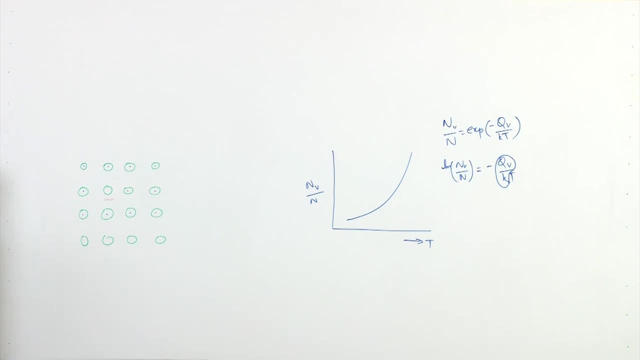 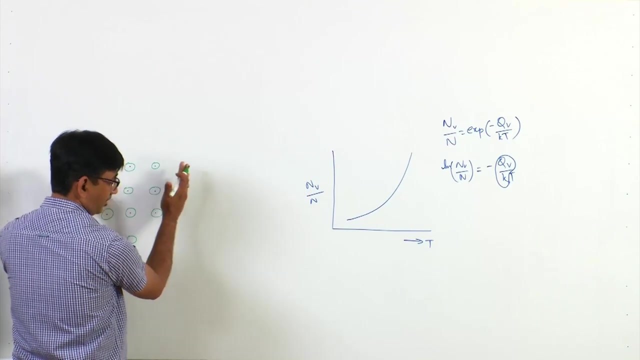 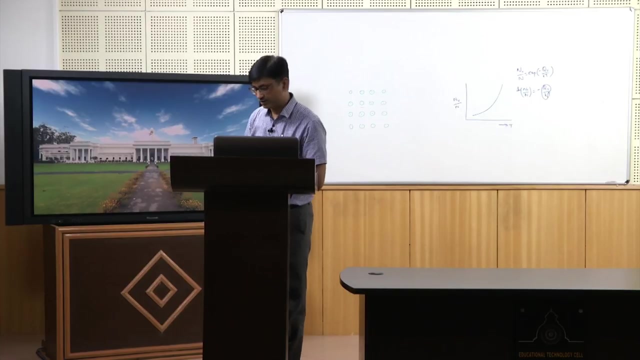 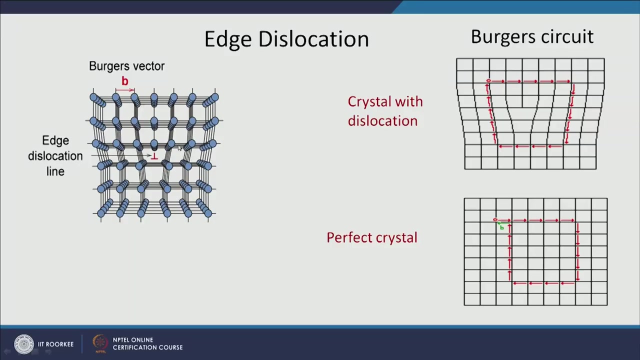 now I have inserted another half plane in that. so what will happen? these suppose I have inserted up to this point. then this atom will kind of give some space for this extra half plane, and that is what is shown here. Wherever the dislocation is ending the, you can see that there is large strain in the. 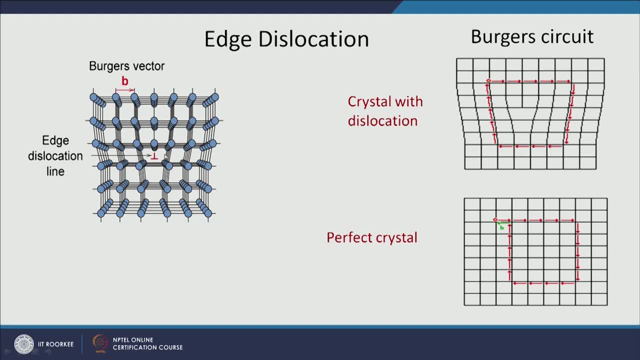 atoms, between the there is a bond length is there and all these bond lengths are stretched. so you have, you are inserting this extra half plane here. after certain distance you will see that all are still nicely arranged on both the side. but where the dislocation 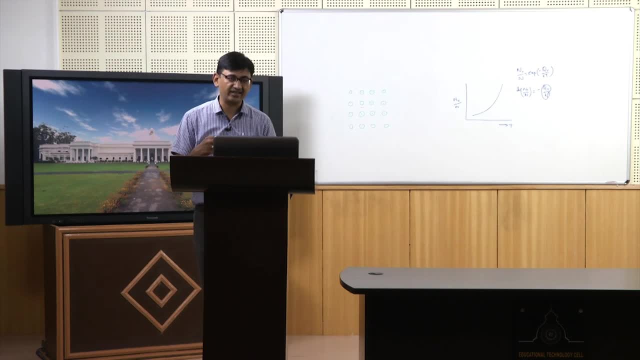 is ending the. there is large number of straining in the material And you can see that this dislocation is going in the direction of the projection here on the slide. so this is the end of the dislocation and it is going in the material like this: 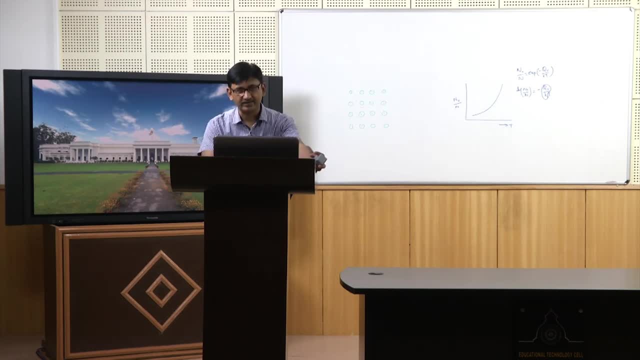 If I want to do see it on a 2 dimension, it will look something like this. now let me define that. what do we mean by the Berger's vector? here you can see that, this one particular slide, this one picture here. 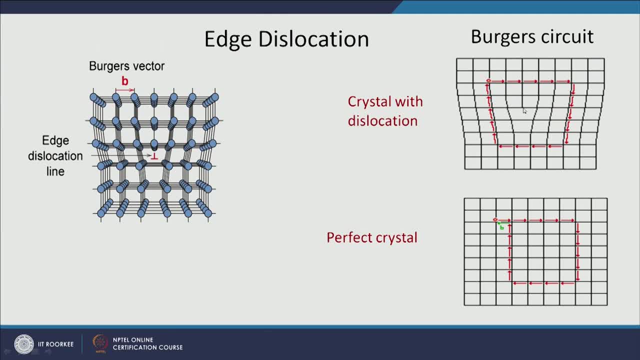 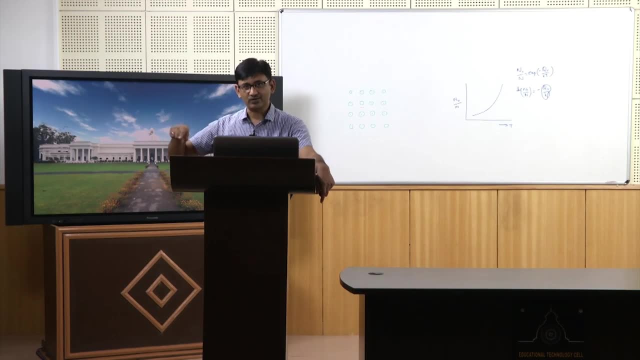 It has a dislocation, a half plane ending here, okay, and the dislocation line is going inside the projection. this is a perfect crystal. okay, so we will take steps. we will roam around the dislocation and see that how many steps are required. okay, so let us we start. 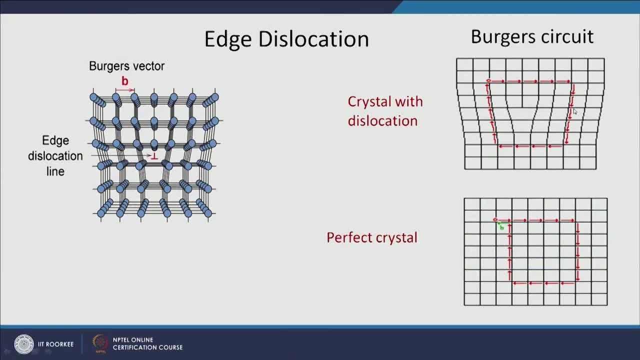 from here: 1,, 2,, 3,, 4,, 5,, 6,, 7,, 8,, 9,, 10,, 11,, 12,, 13,, 14,, 15,, 16,, 17,, 18,, 19,, 20,, 21,, 22,. 23,, 24,, 25,, 26,, 27,, 28,, 29,, 30,, 31,, 32,, 33,, 34,, 35,, 36,, 37,, 38,, 39,, 40,, 41,, 42,, 43,, 42, 43,. 45,, 46,, 47,, 49,, 40,, 42,, 45,, 46,, 49,, 40,, 42,, 45,, 46,, 49,, 40,, 42,, 45,, 46,, 49,, 40,, 42,, 45,. 50,, 51,, 51,, 52,, 52,, 52,, 53,, 53,, 53,, 53,, 54,, 54,, 55,, 56,, 56,, 57,, 57,, 58,, 59,, 90,, 90,. 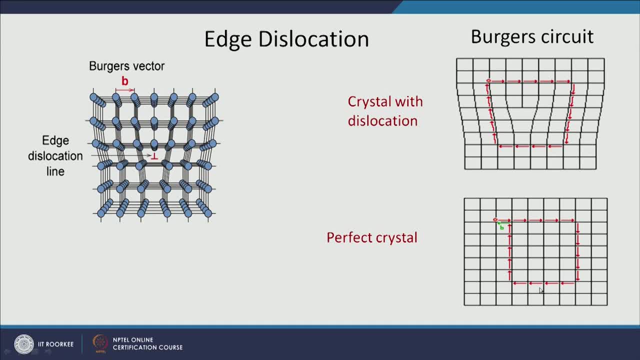 20. okay. Now, same thing we will do here. okay, as we have done, we are starting from the same position, we are going along taking the same steps, okay, and we will find that we are reaching early here. okay, so extra step which we took here because of the extra half plane we are 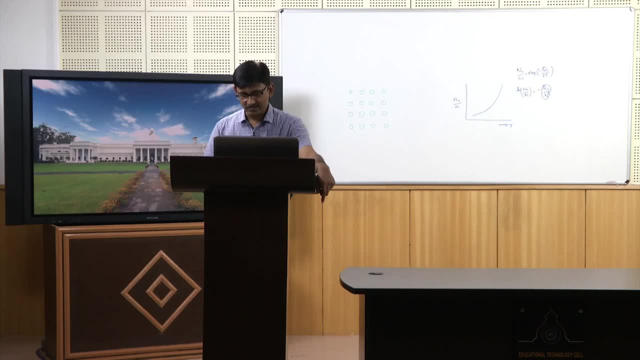 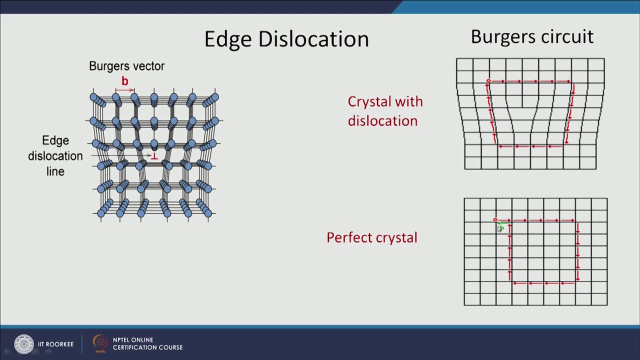 not going to take in the perfect crystal, okay, so this extra distance which we are travelling in the crystal which contains dislocation, that is going to give me the Burgers vector, okay, So this is my extra half extra length which I have travelled, which is equal to this atomic. 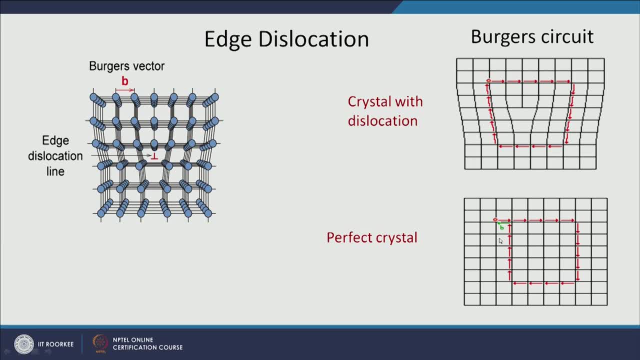 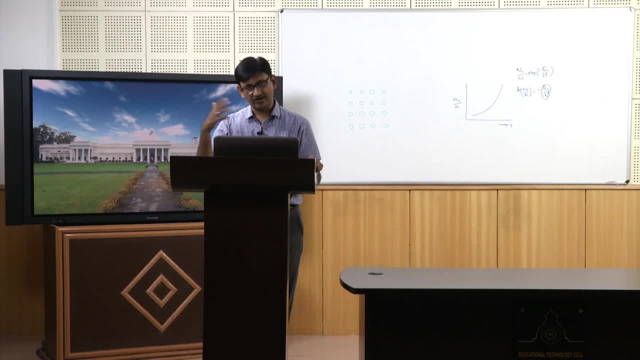 spacing here and that is equal to B. okay, that is the Burgers vector. So by using Burgers vector I can define that. what type of dislocation is this in another plane? the Burgers vector? Burgers vector will be different because the atomic spacing will be different. okay, 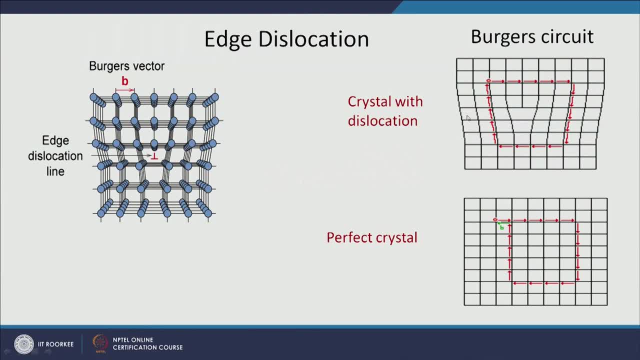 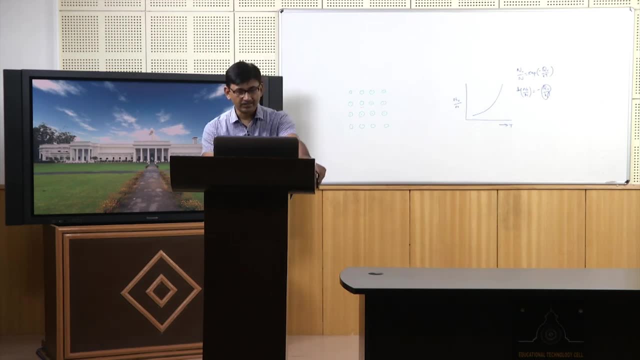 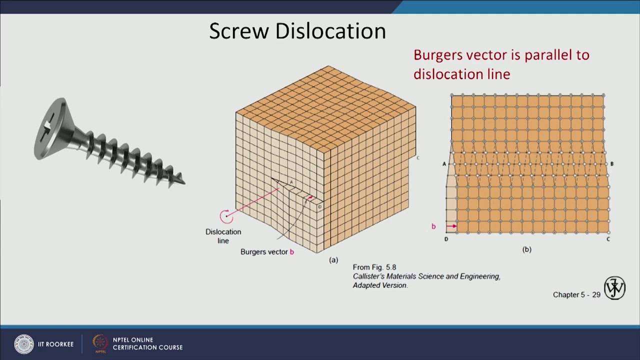 so this is how the edge dislocation will look like and this is how, by drawing a circuit around the dislocation and a perfect crystal, I can find out that what will be the magnitude and the direction of Burgers vector will be okay. Similarly, in a screw dislocation- actually the visualization is slightly difficult because 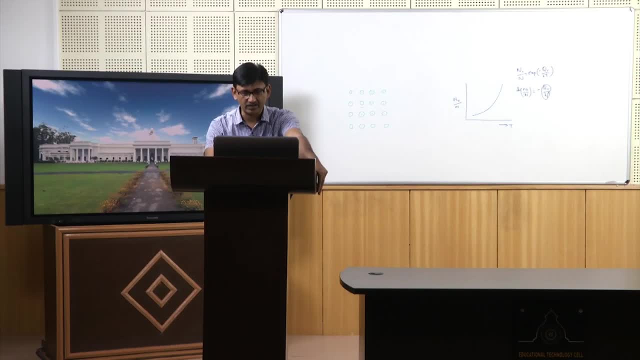 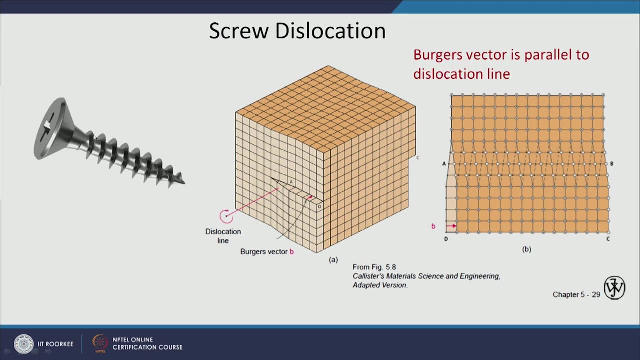 it is a 3 dimensional movement of atoms around the dislocation. okay, you can see it from a screw kind of geometry. okay, so if I am moving from this particular side and going along the screw, okay, so I will go down and then from the back I will come somewhere here. 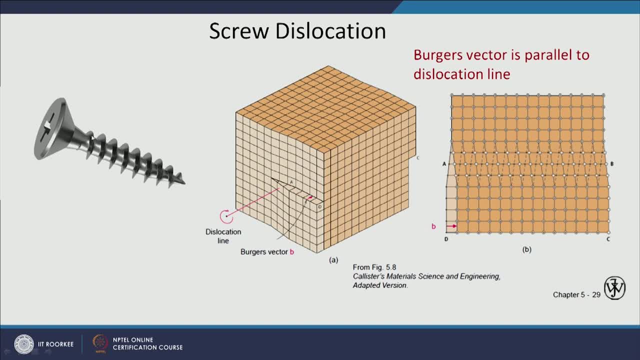 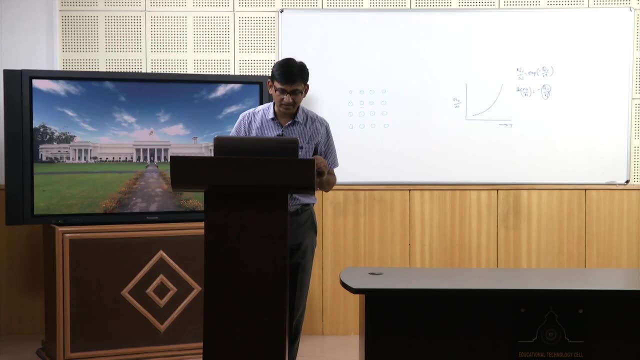 okay. so when I am moving like this, I have moved by a pitch of the screw, okay, as a mechanical engineer, So this is what we call as pitch of the screw. so I have moved by a pitch of the screw, okay, in which, in case of dislocation, is the Burgers vector. 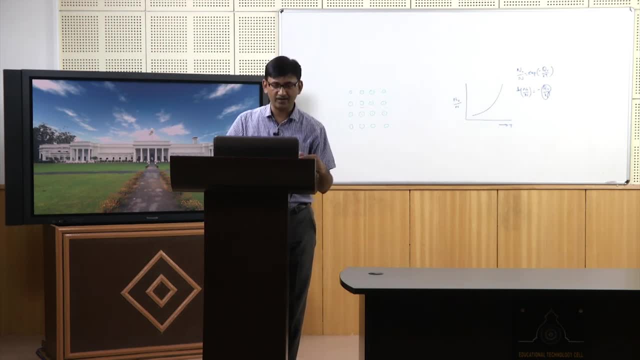 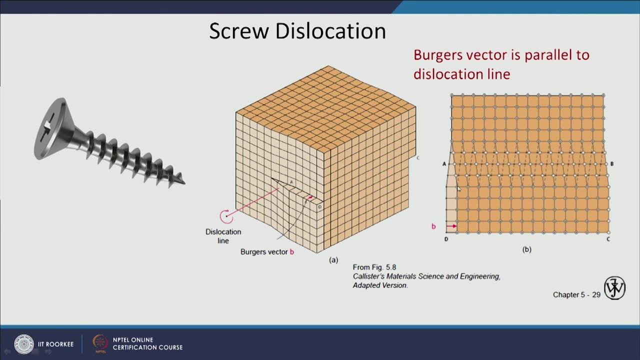 So while I am taking this one rotation, I have moved by one Burgers vector here. okay, and that is what is shown here: that if I this is the open circle and the closed circle small. the atoms are shown in the circle, Okay. Okay, So in the lower plane and the close open circle are shown on the upper plane. okay, so in this. 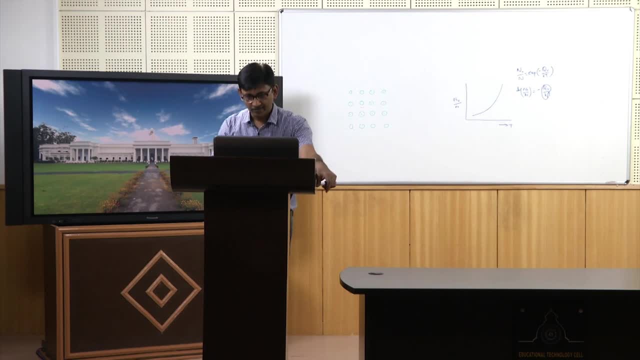 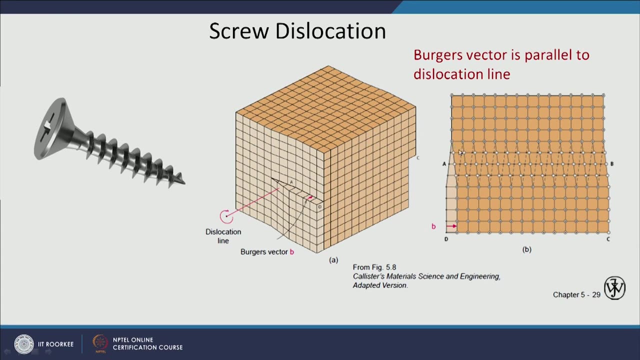 two location. they are one above another, but where the dislocation is, they are displaced by a small distance. so when you travel one whole distance, you will create a dislocation of one Burgers vector. okay, so this is what we call as screw dislocation. so one is edge. 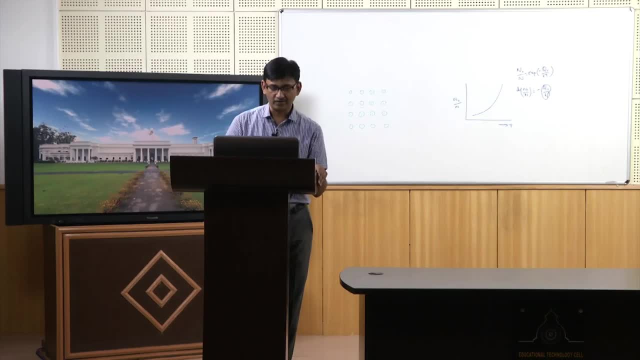 dislocation. Another is screw dislocation. okay, you do not have to worry about too much about this classification. only thing we have to understand here is that dislocations are there in material, okay, and they help in the deformation process. by doing this slip of two atomic planes by 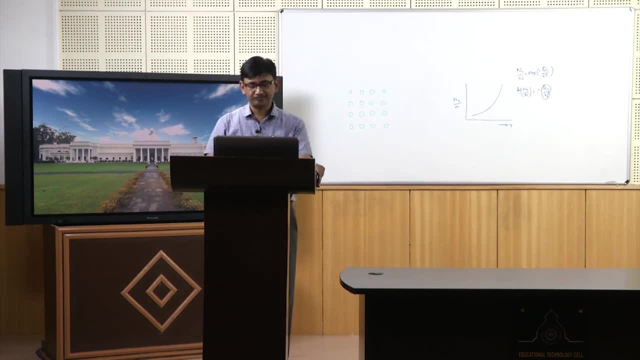 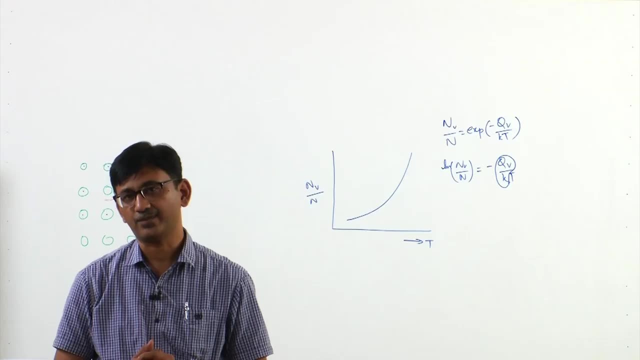 in steps rather than in one step. okay. Then the next one, which is of importance, Okay, Okay. So this is already we have seen and we have discussed about grain boundaries. okay, this is a planar defect, means it is over an area, okay. 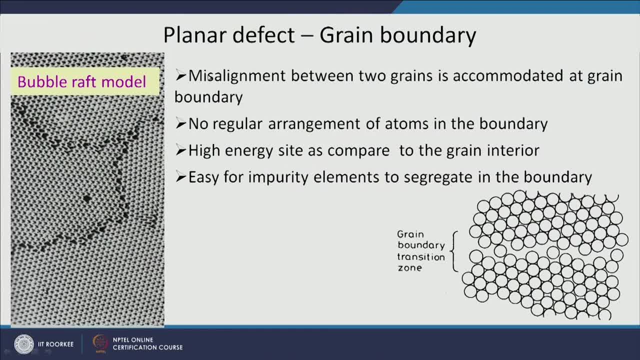 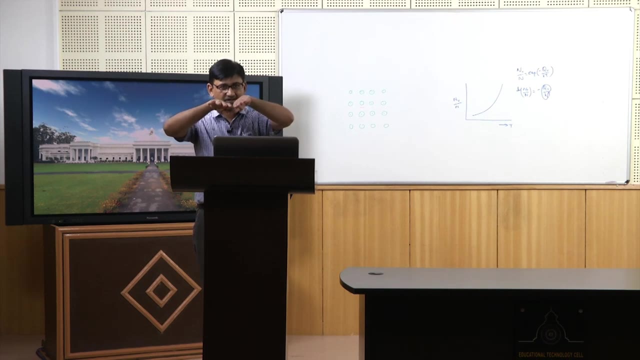 So, basically, what grain boundary does, is it kind of accommodate the misalignment between two grains, as you can see that there is a nice atomic arrangement here, okay, in one direction. in another grain also, you can see a very nice atomic arrangement is there Okay. So if these two arrangements are meeting, okay, because their alignments are different, okay. 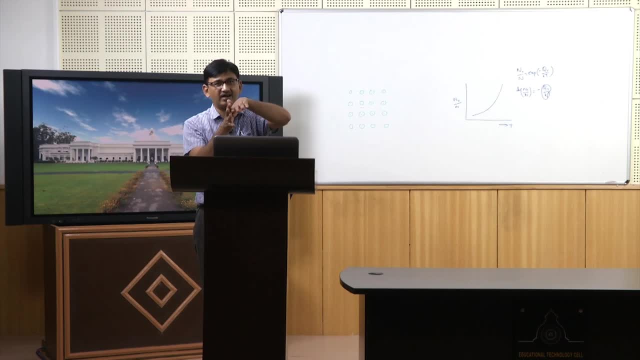 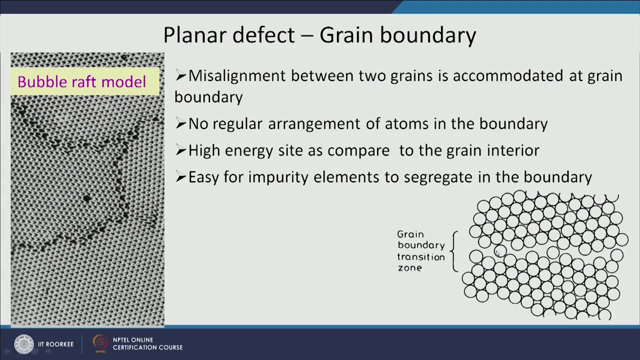 I have to have some kind of an area where the misalignment can be accommodated and then the new alignment will start. okay, and that is what is called as boundary. in this case it is because between two grains you call it as grain boundary, And where you have grain boundary you can see that the arrangement of atom is not regular. 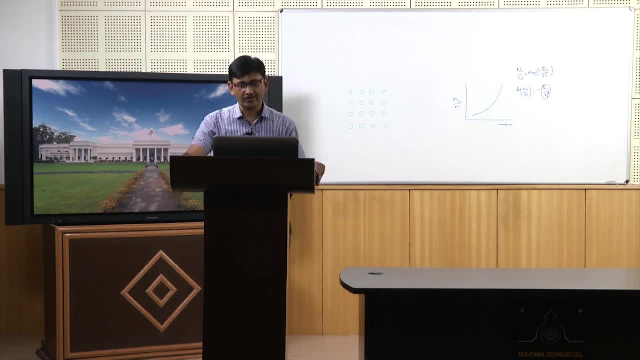 as in the grains Or as in the crystals, okay, and the bond lengths are also are not of equilibrium distance, they are kind of stretched. So you can also understand that these are high energy areas because the bond length is not at their equilibrium distance. okay, and also, you can see, because there are more. 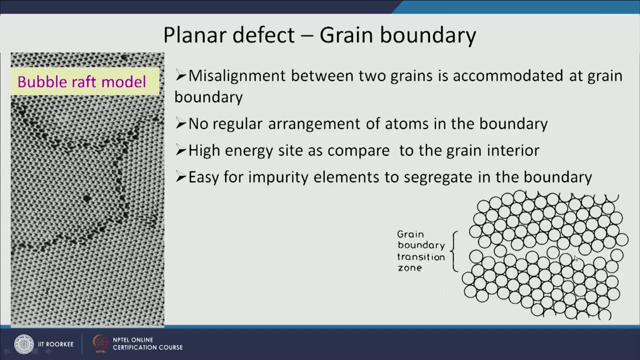 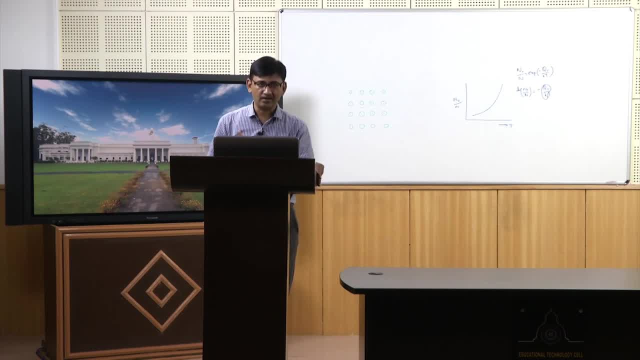 gaps available here for any impurity atom or foreign atom to come and sit here, is very easy for it. okay, so there is a segregation of atoms. okay, in the grain boundary. So whenever you have foreign atom, sometime you are alloying, making an alloy for those. 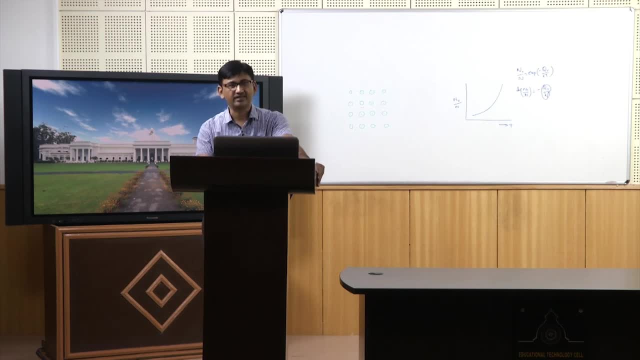 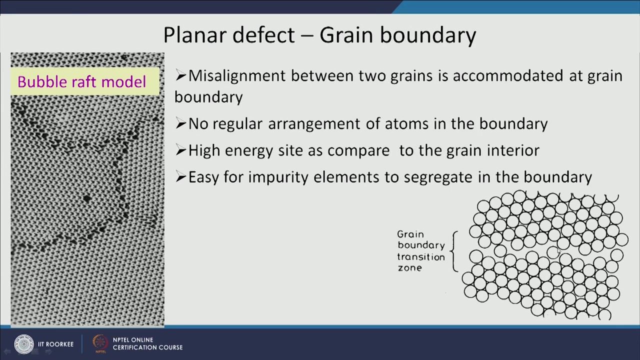 alloying element. it is very easy for them to come and sit at the grain boundary okay, which we usually do not want, but because there are large number of gaps in the boundary that is, So you can sit in this boundary sites okay. a nice kind of analysis people have done about. 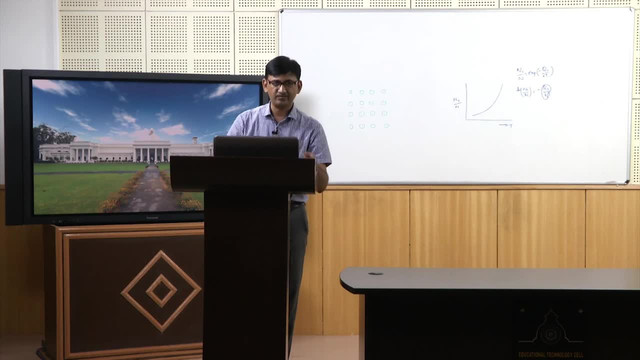 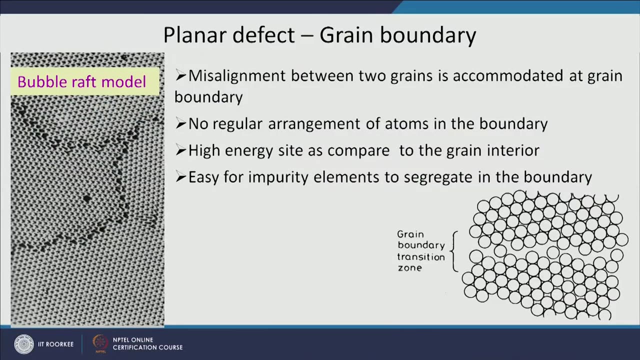 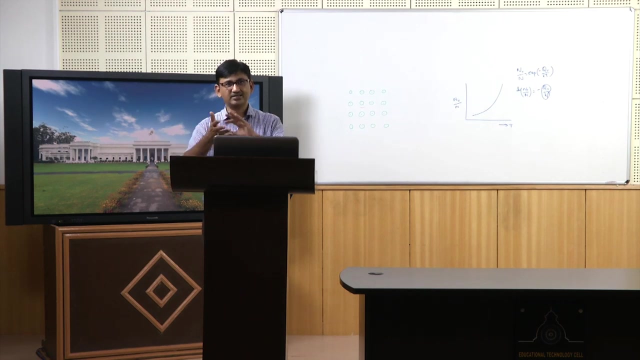 grain boundaries by this kind of bubble raft model. Bubble raft means these are soap bubbles, okay, which are arranged in a three dimensional area or space, okay, and those areas are photographed. you can see that in these bubbles also some arrangement will be there. So you can see, there will be a nice arrangement and suddenly somewhere there the arrangement. 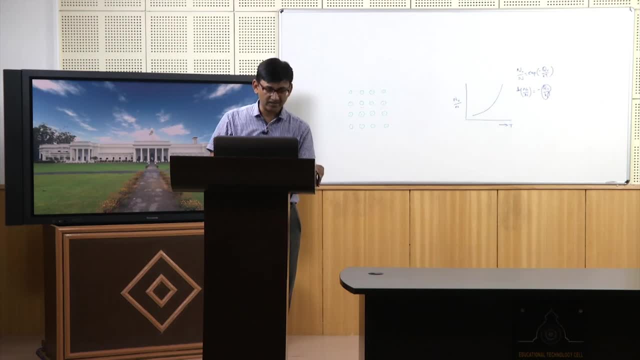 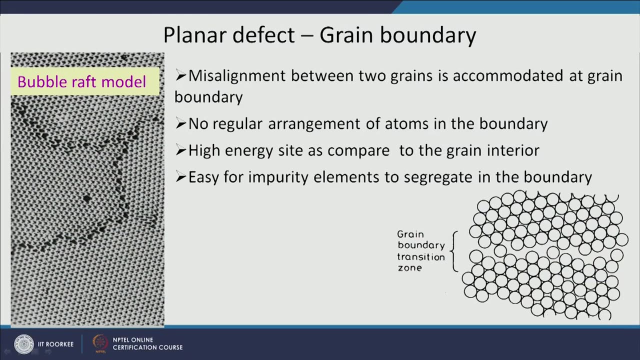 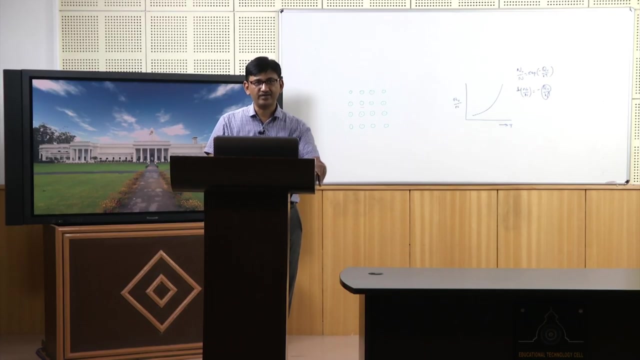 will break and the next arrangement will start. so you can see that this will be a nice arrangement. it will look like a grain, okay. but in this part there is another arrangement coming and this will be the boundary which is accommodating the misalignment between the two grains. 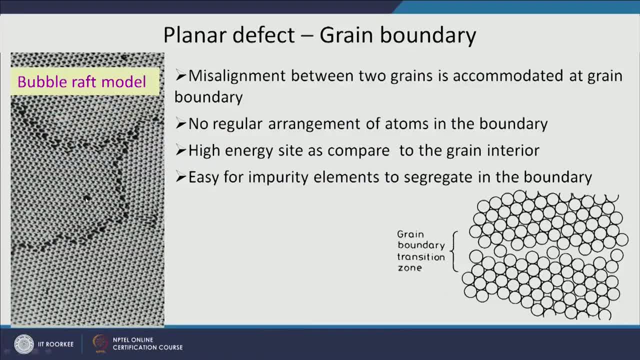 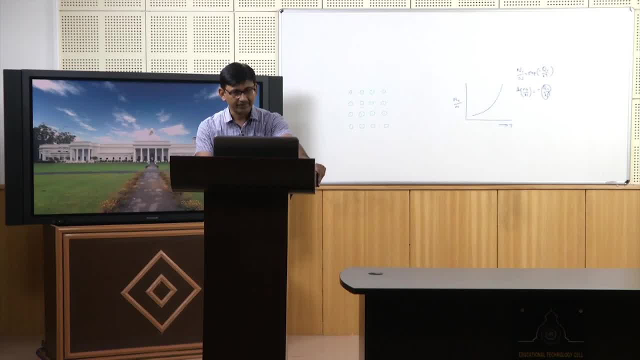 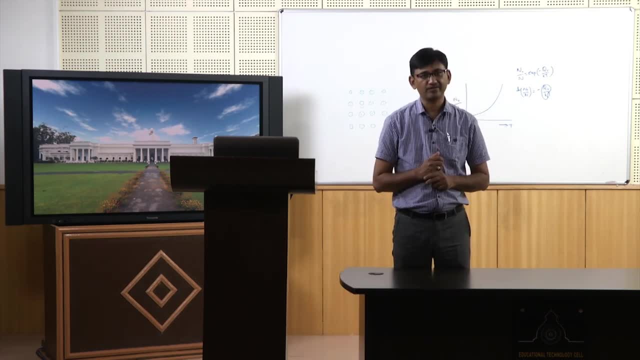 One. another interesting thing you can see here is that there is a vacancy here. that means The boundary is missing from this side, so there is a vacancy also here. okay then, there are some special type of boundaries are also there in this case, one of the boundary which. 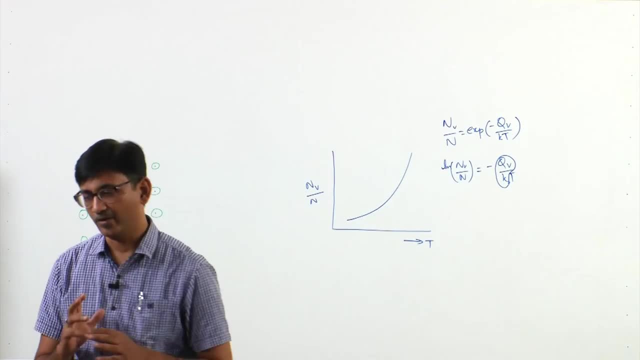 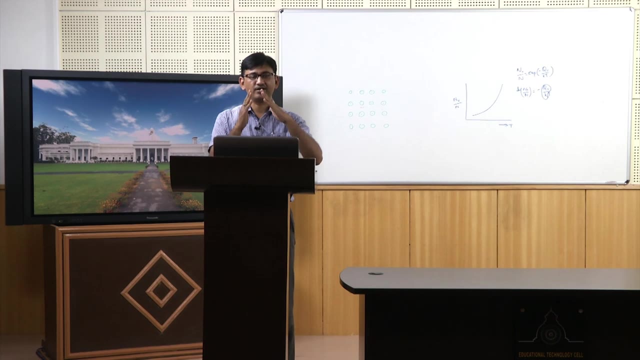 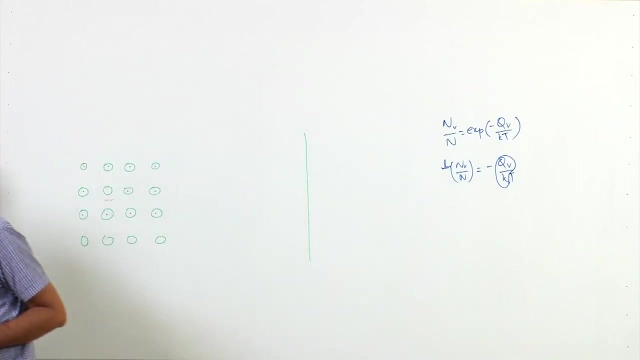 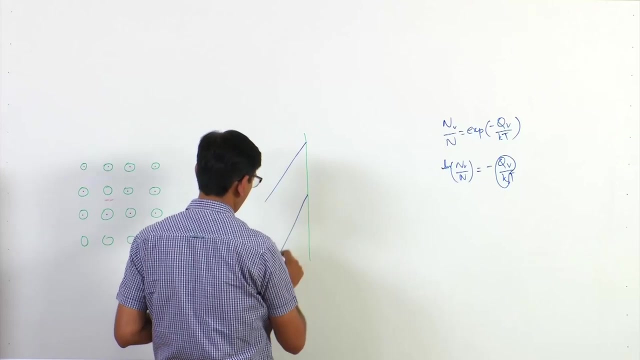 we have is called twin boundary. okay, so the twin boundary, as the name suggests, you can understand that it has a mirror kind of arrangement across the boundary. okay, so suppose in one grain The arrangement is like this: okay, so suppose this is my boundary. okay, and this is, for example, 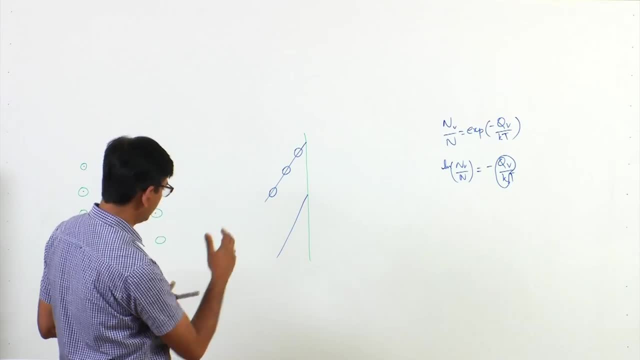 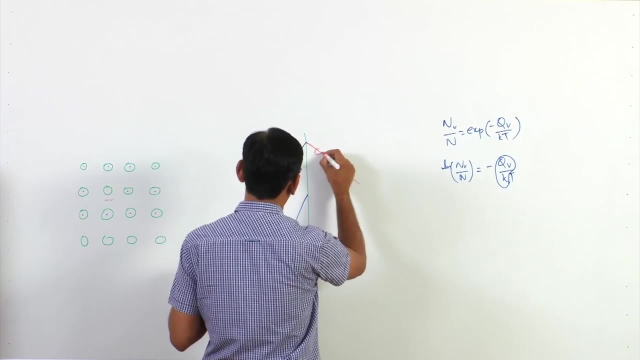 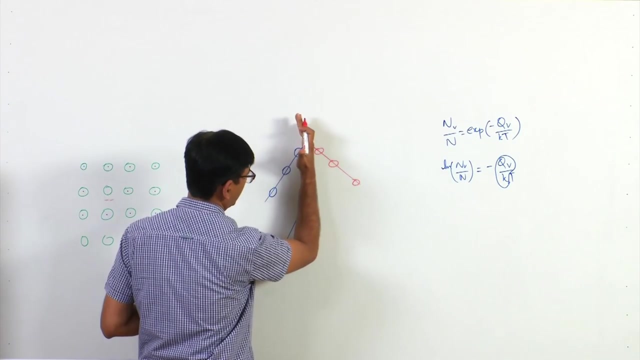 atoms are arranged like this. okay, so if you see this thing in mirror, how you will see it? this atom will be mirrored here, this atom will be mirrored here, this atom will be mirrored here. So it looks like that there is a mirror here and all these atoms are. there is a reflection. 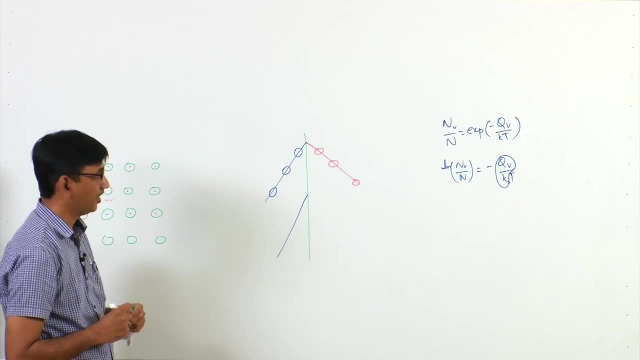 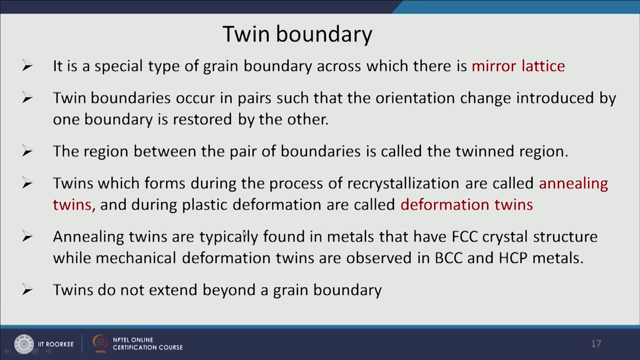 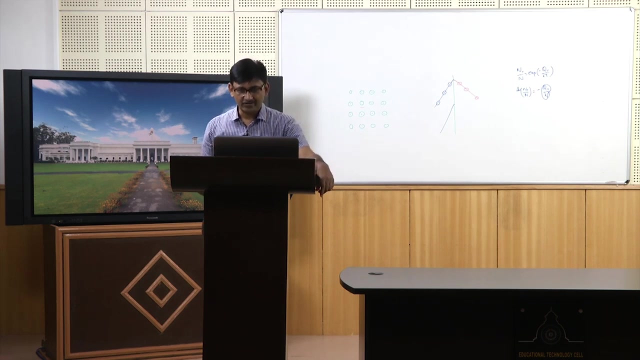 of these atom across in the mirror. okay, and this kind of boundaries are called twin boundaries, which has a mirror like of arrangement of atoms across the boundary. okay, Some other properties of twin boundaries are that usually, not always, they occur in pairs. so Let us say two boundaries together, okay, so whatever change in orientation is there. so 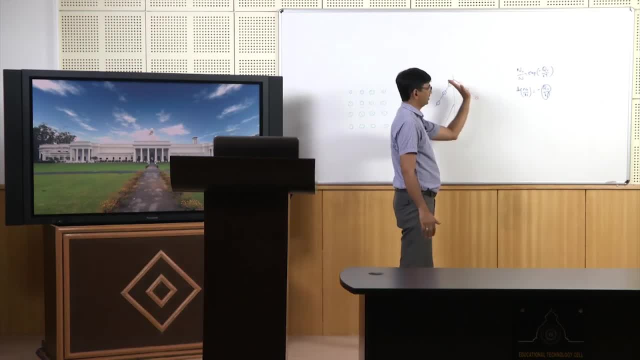 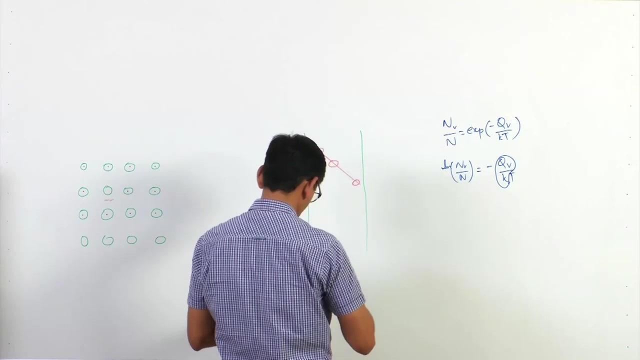 you can see that this is this arrangement. and then there is a another type of arrangement. so when another boundary comes, it will again become the same arrangement as this one. for example, if I put another boundary here, okay, so across this it will again become. this will be reflected here. 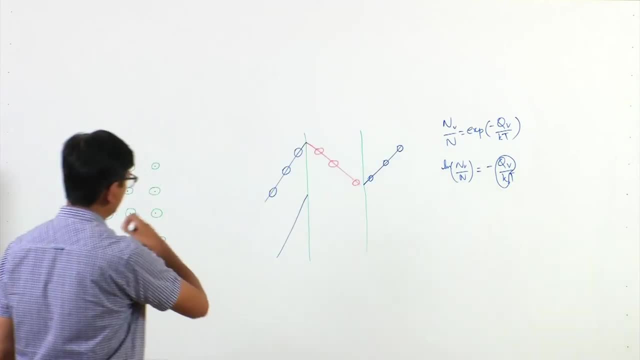 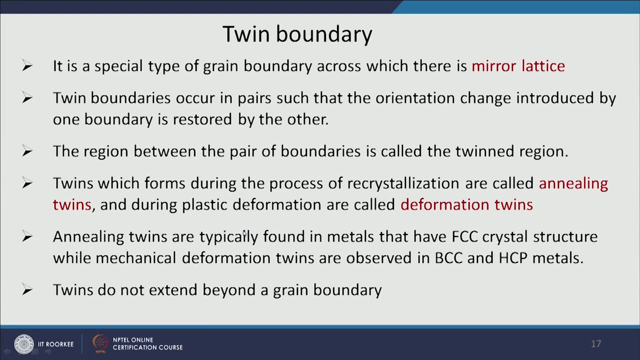 So you can see the arrangement is again coming back to the original arrangement. okay, so if you have two boundaries together, the orientation change introduced by one boundary is restored by the other. the region between the pair of boundaries is called the twin region, so this area will be called the twinned region- twins, which form during the process of recrystallization. 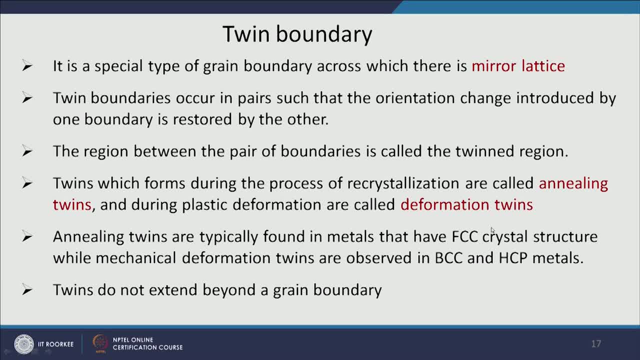 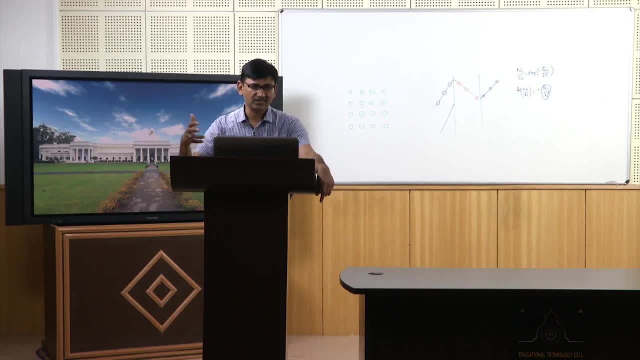 are called annealing twins And, during plastic deformation, are called deformation twins. okay, annealing twins are typically found in metals that have FCC crystal structure, while mechanical deformation twins are observed in BCC and HP metals. So you can understand that all these features are also dependent on the crystal structures. 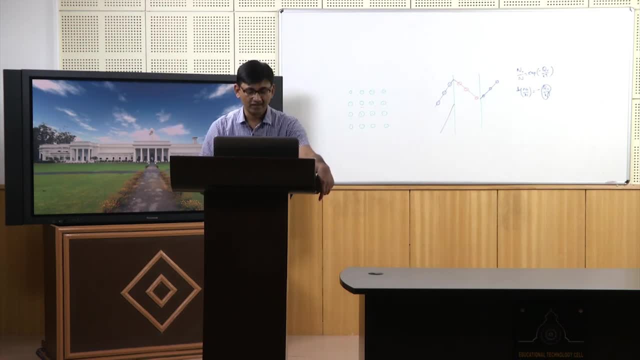 which we studied in the beginning. okay, Twins do not extend beyond a grain boundary. okay, so a grain boundary will be the kind of a limiting For a To go beyond that. okay, So, if you remember, I showed you this kind of twins earlier, also in the same micrograph. 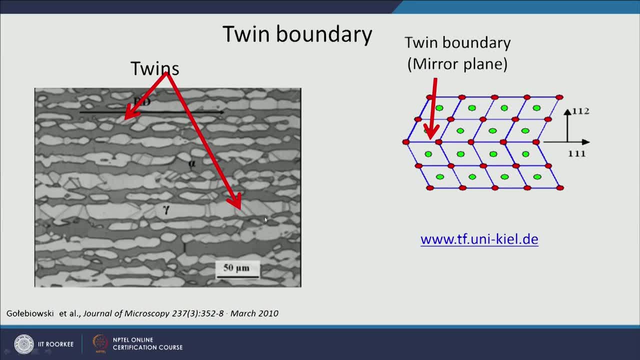 you can see that these two twins are coming in pair okay. there are other location also where the twins are coming in pairs okay. For example, here they are coming in pair- okay, and you can also see that they are not going beyond their particular grain boundary. 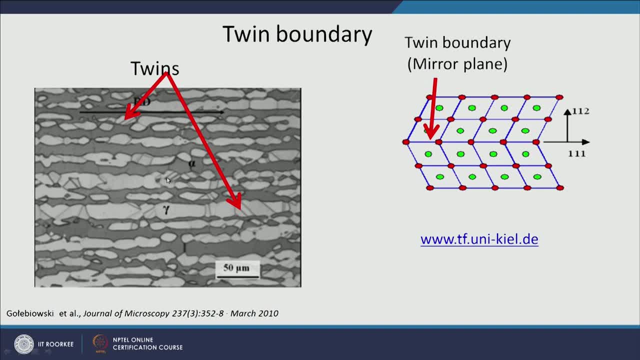 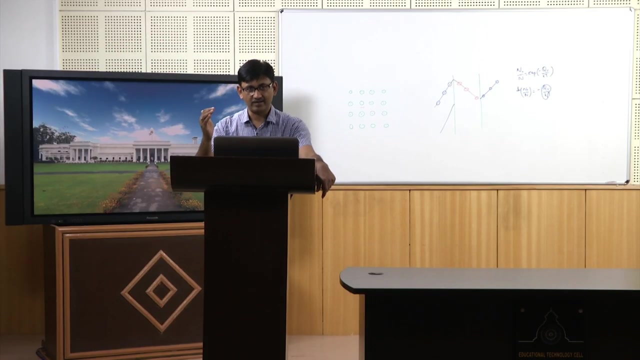 So they are starting from here, ending here. okay, so it is not going beyond this particular grain boundary here. okay, this also you can see, because anyway, there is another phase coming, so it will not go beyond this particular phase boundary here. okay, So the phase boundary or the grain boundary will be the limiting where it will not go. 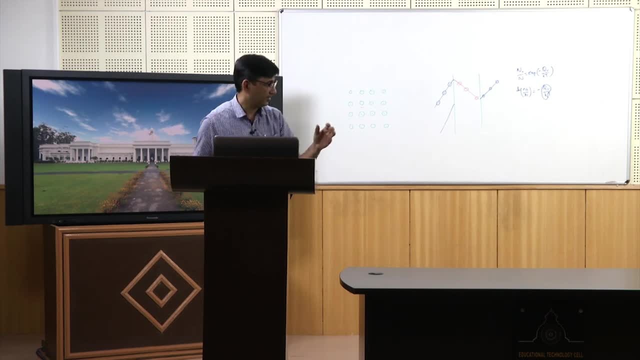 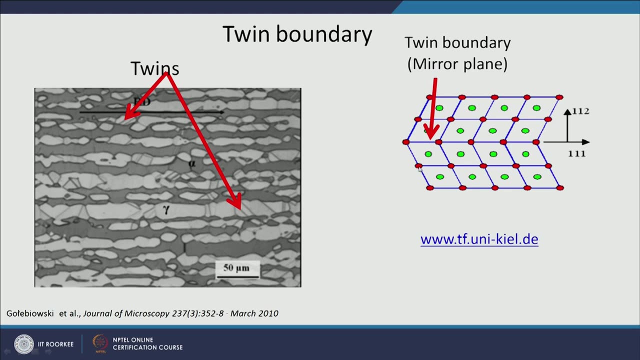 beyond that, You can see the idea which I was talking about earlier. Yes, Take a look at this. I was telling you there. okay, this is my boundary, and this particular atom is mirrored here, this one is mirrored here, this one is mirrored here, and so on. 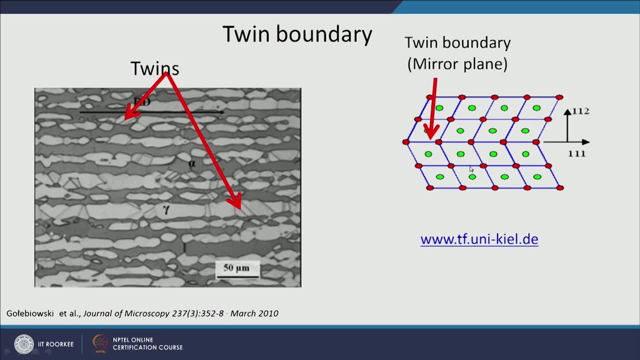 So it looks like a mirror boundary and the atoms on both the side look like a mirror image of each other. okay, So these are called twin boundaries. these are special type of boundaries. it will not be very commonly seen, okay, but in certain situation it will be very prominent, as you. 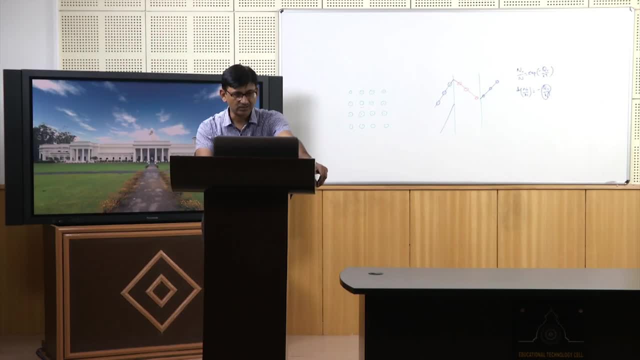 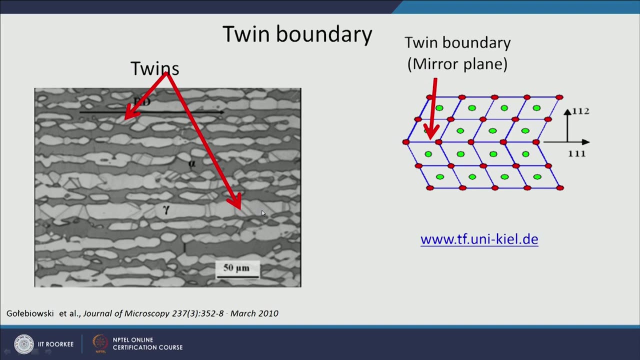 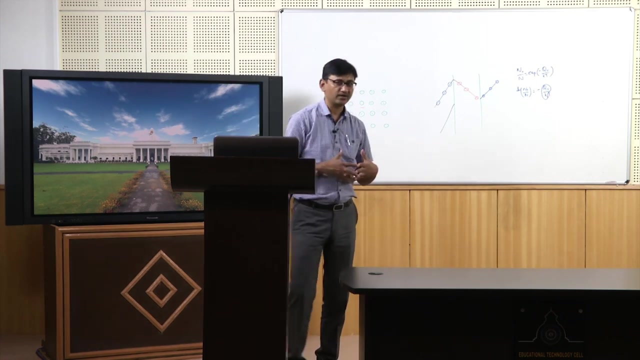 can see in this particular case. so in alpha phase, which is BCC crystal, you will not see any twin. but gamma phase, which is an FCC, you are seeing lot of twins, okay, in the same material. So with that, this is about defects. okay, so we have seen point defects, line defects and 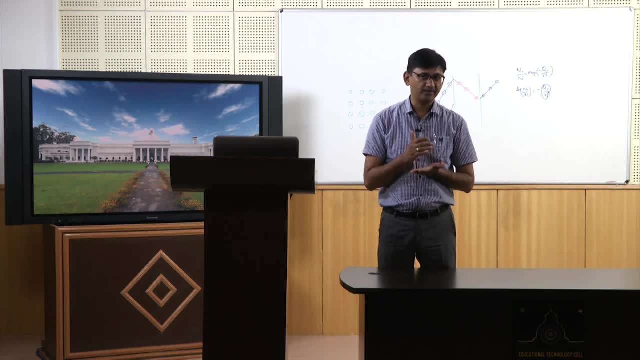 area defects: Line defects: the dislocations are a very important defect to understand because lot of properties depend on them. similarly, grain boundary is a very important defect because grain boundary actually limits the how much the dislocation is going to move. okay, which we will see later on. also okay.